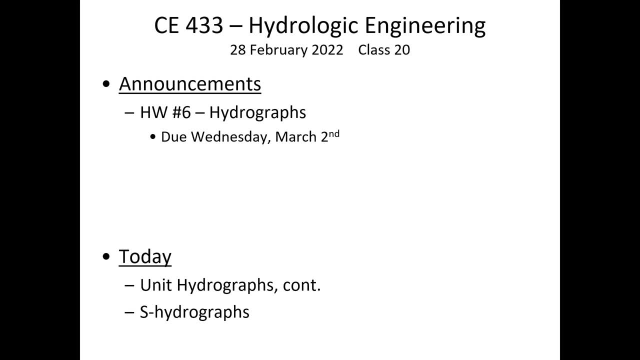 hydrograph. What is it predicting? The flow in a stream? Yeah, so flow rate. So we think of it as a model, Just a way of representing reality, And what goes into the model is rainfall excess, if we're being precise about it. And then what comes out of the model is runoff in a stream, So unit 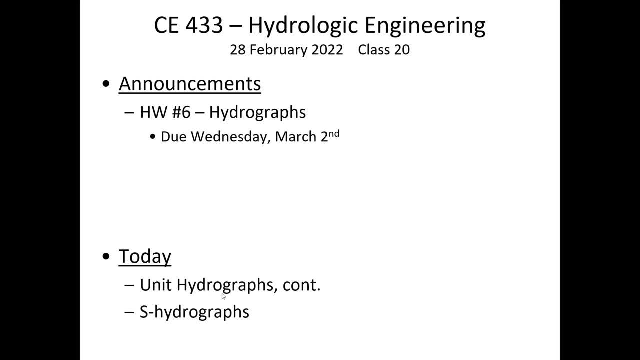 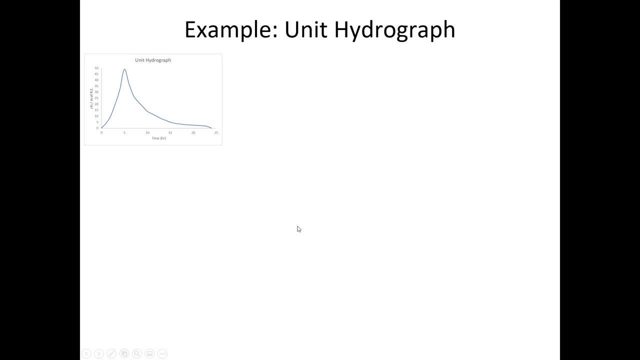 hydrographs. We have an example that illustrates that and then something called an S hydrograph. We're going to go over both of those today. So just to make that point visually, let's say that we have units here, And maybe that's a bit small for you to see, but on the horizontal axis it says: 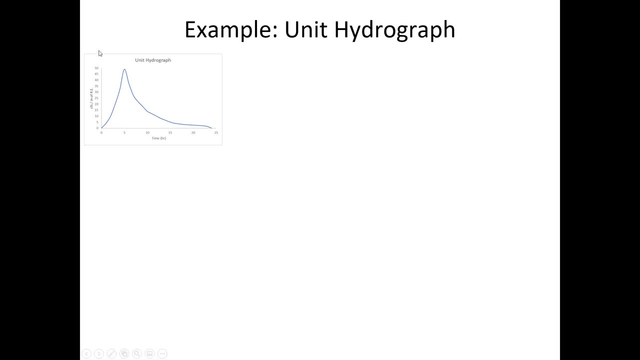 time in hours, And what generated this unit hydrograph was a certain amount of rainfall excess in a specified time period, And so in this example, we're going to say that it was 1 inch of rainfall excess in a 1 hour period, But you could also make a unit hydrograph that shows what would be. 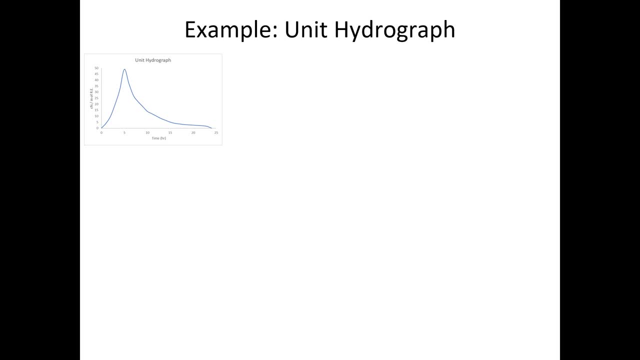 watershed response for an inch of rainfall that falls in a four-hour period, And so there are different storm durations and just to I don't know skip ahead a little bit. the purpose of the S-hydrograph method that I'll show in the second half of today's class is: 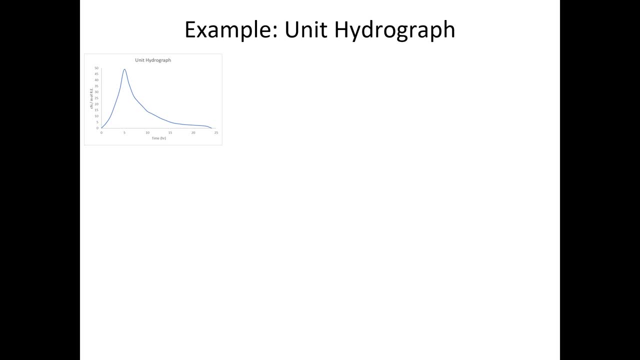 to adjust the duration of the storm, So it doesn't always have to be a one-hour storm duration that generates a unit hydrograph. But for this first example, we're going to assume that an inch of rainfall excess causes this response. Now, this response is only. 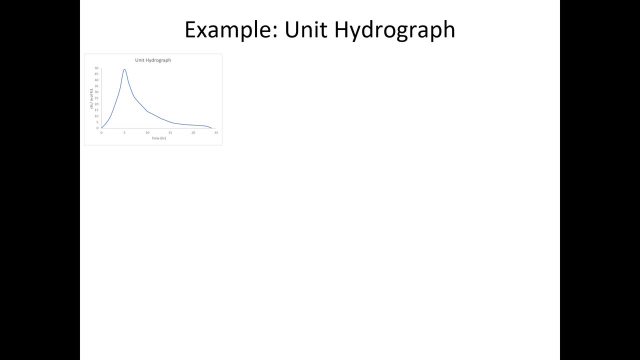 going to be valid for the watershed in question. So our particular watershed may have a certain area, a certain basin, slope, sinuosity, It may have certain vegetative and soil characteristics, And so it's completely unique And you couldn't take this unit hydrograph and transfer it. 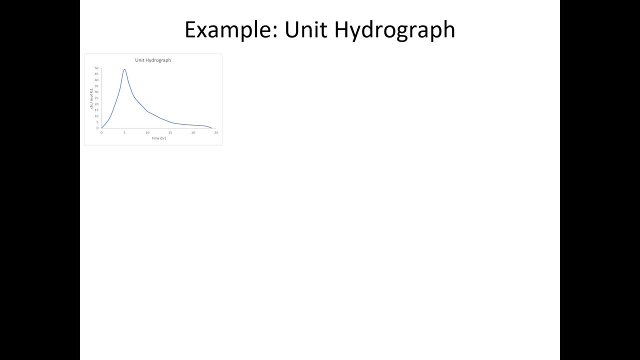 exactly to another spot, although you could make adjustments And maybe try and adapt it to a different location. But a unit hydrograph that's generated from pure observation only applies to its watershed. And then think again also: what were the antecedent moisture conditions when this unit hydrograph was generated? In other 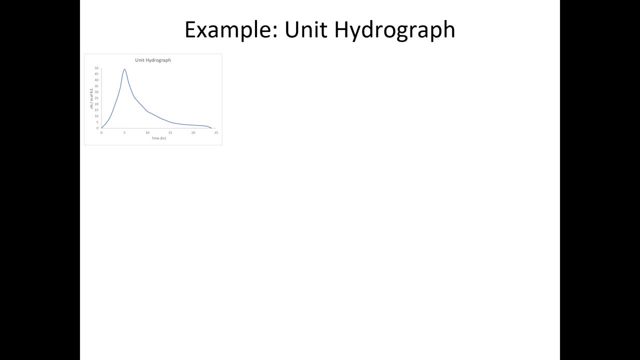 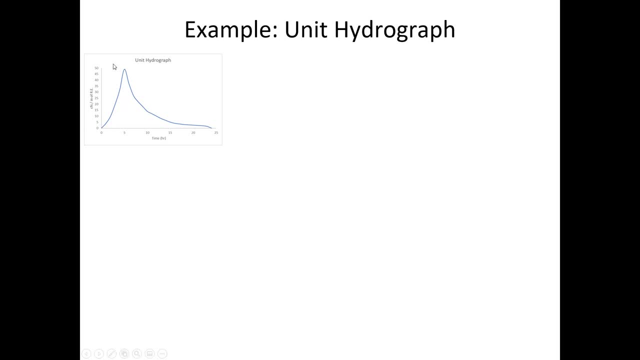 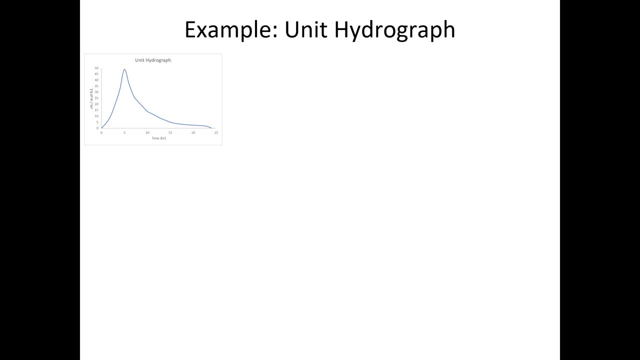 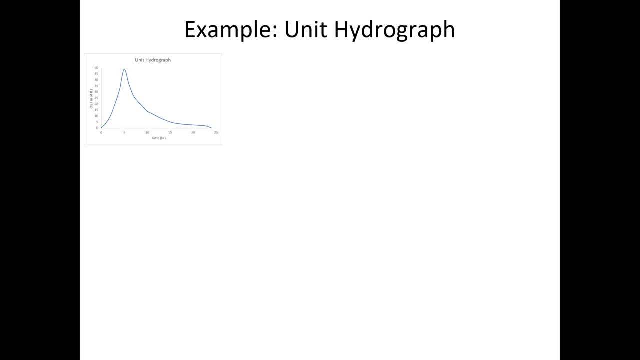 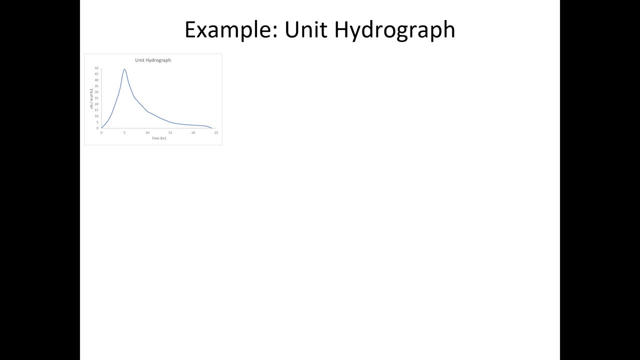 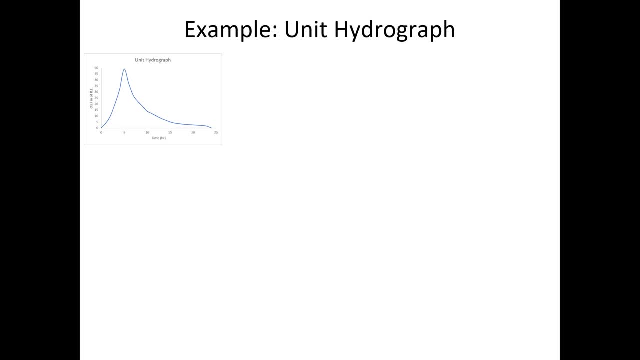 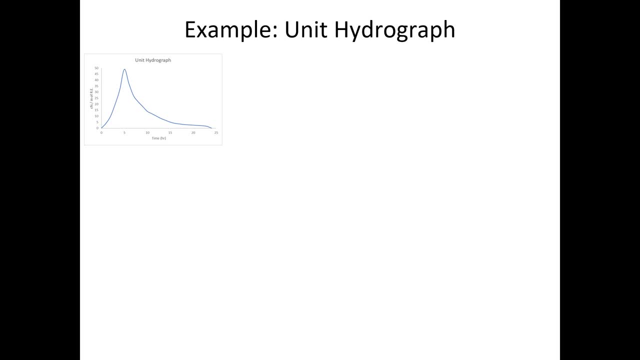 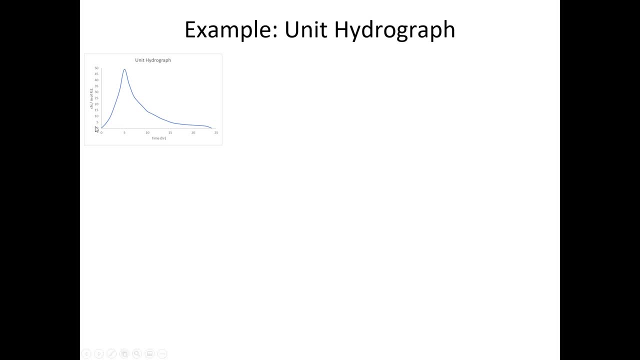 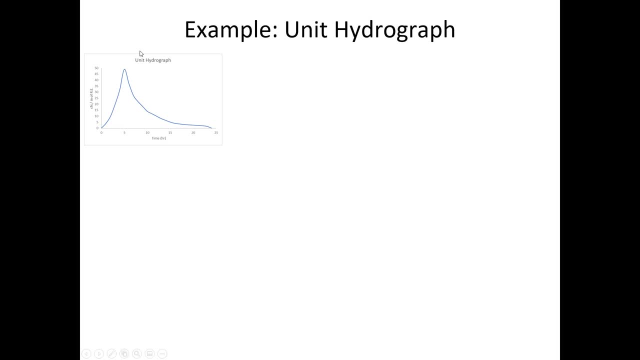 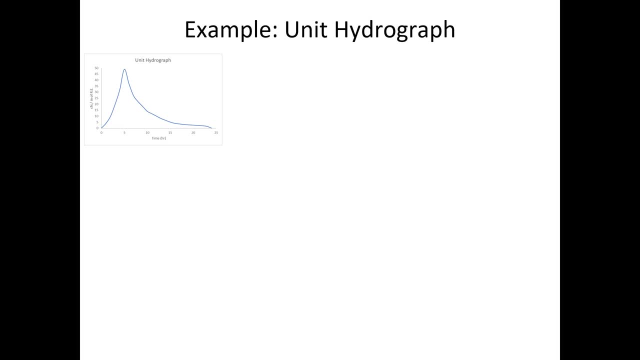 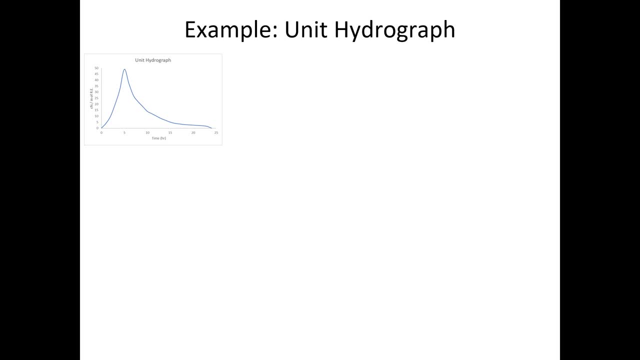 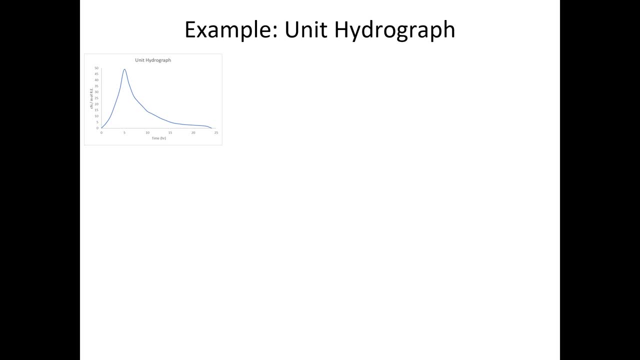 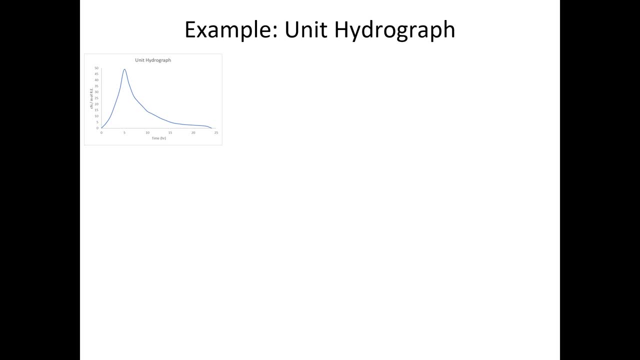 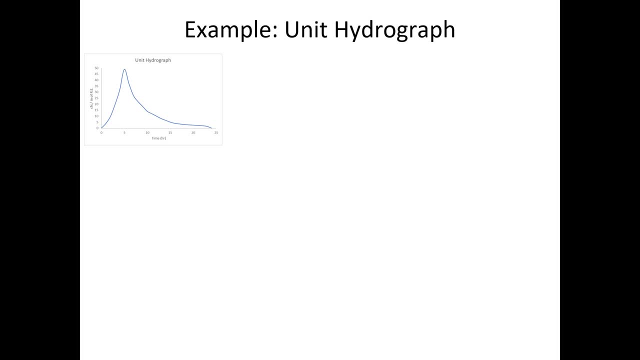 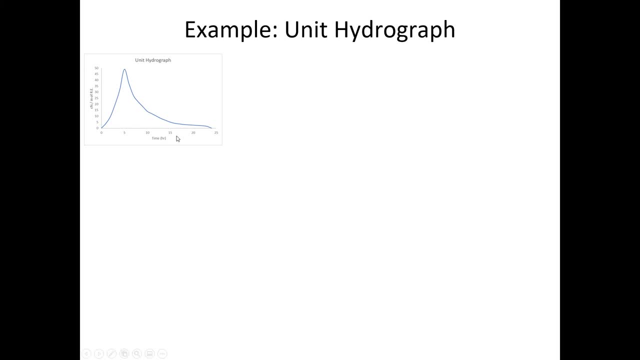 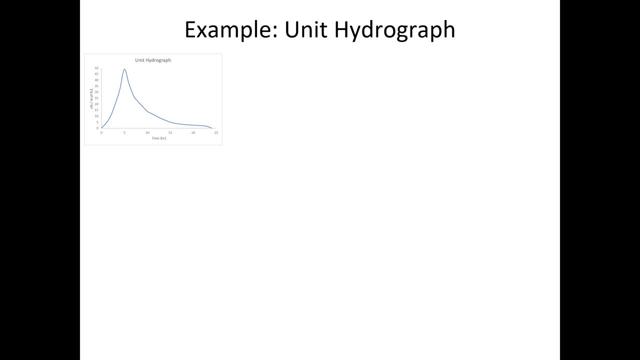 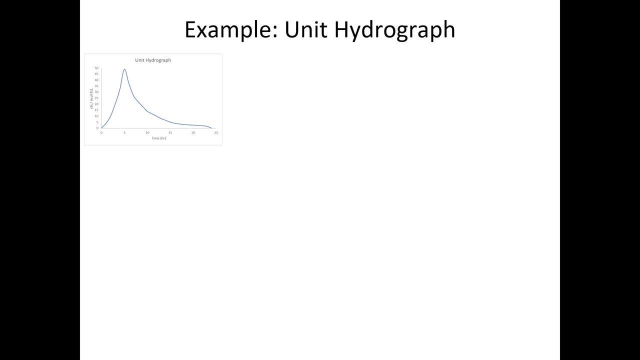 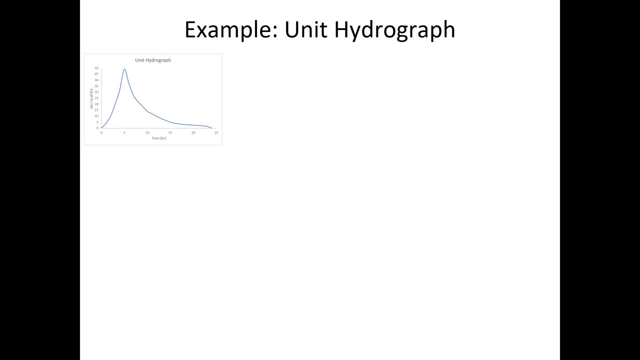 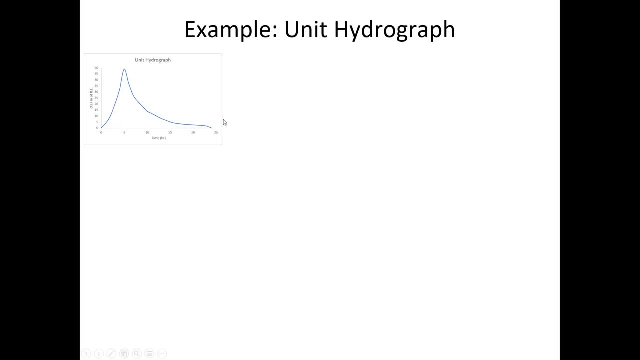 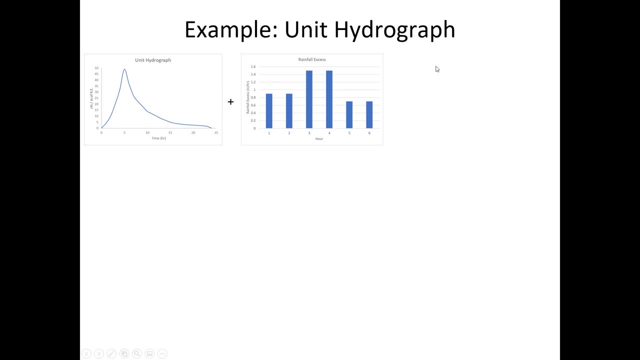 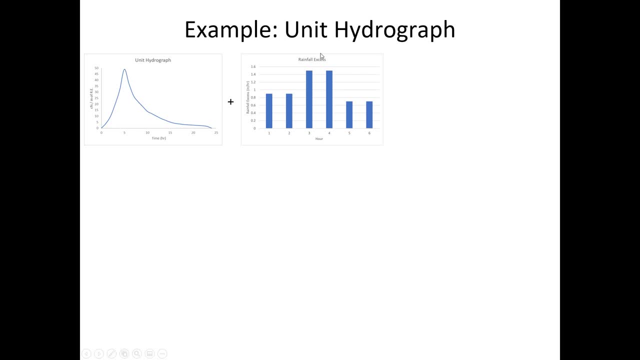 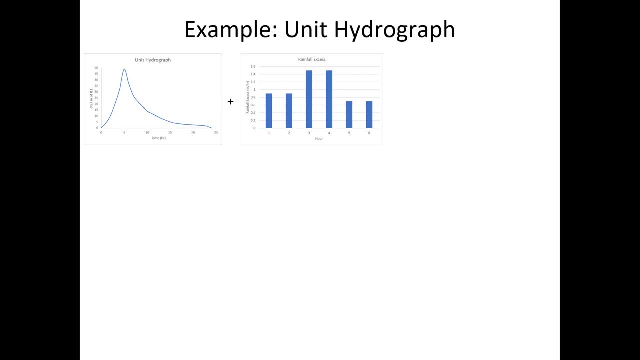 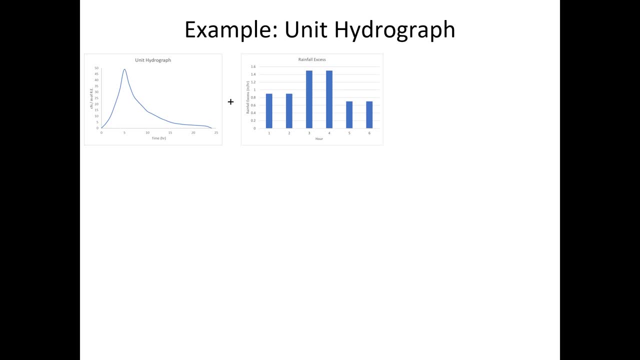 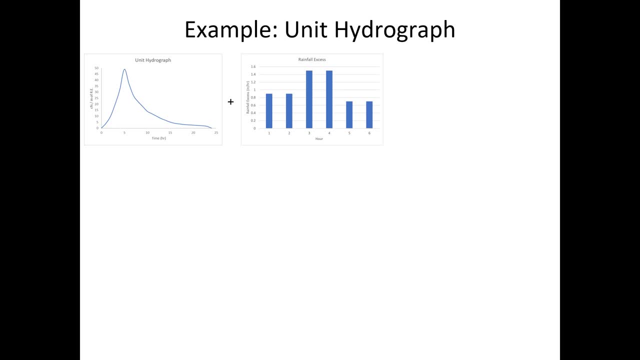 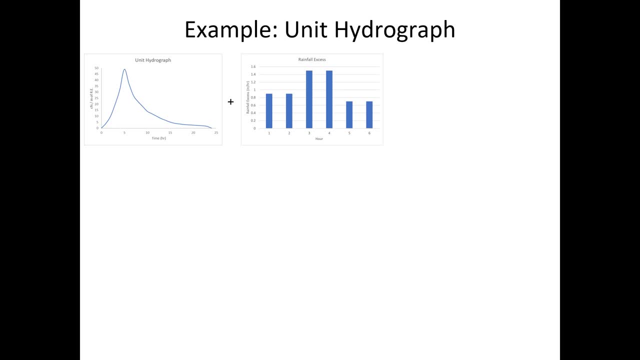 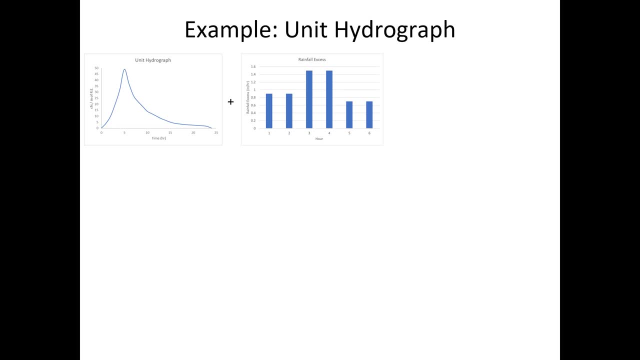 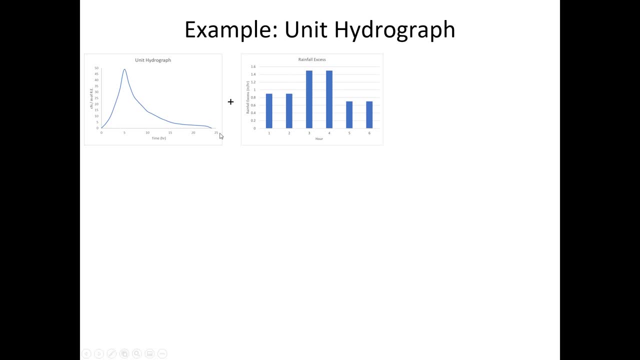 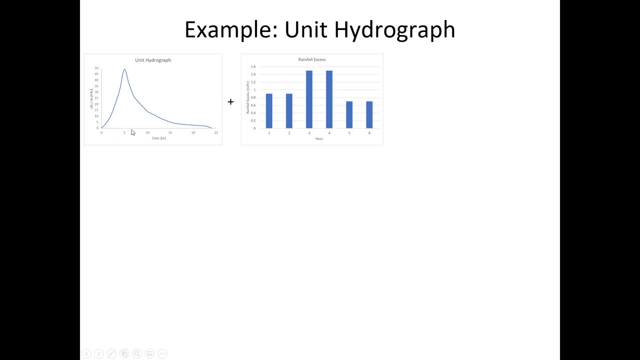 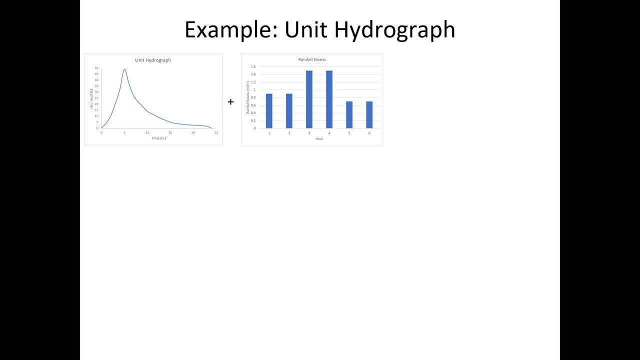 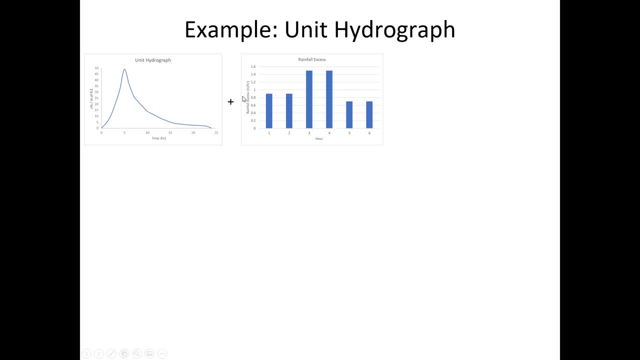 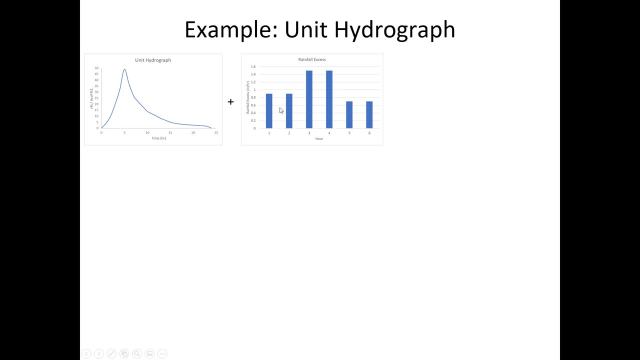 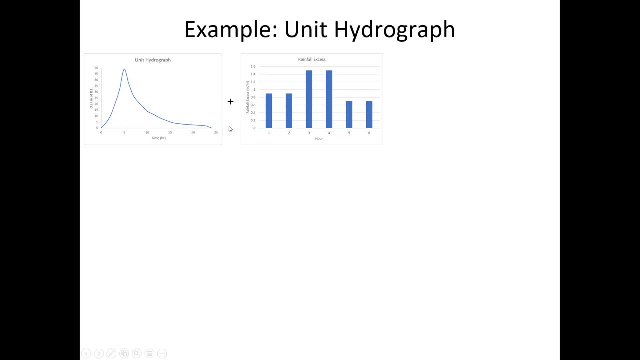 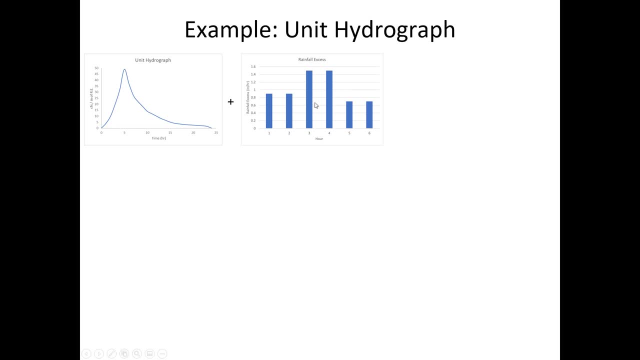 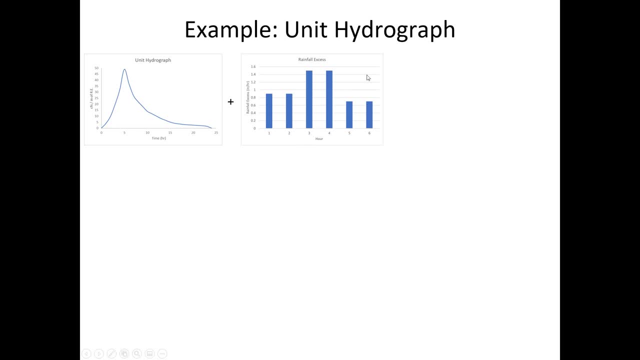 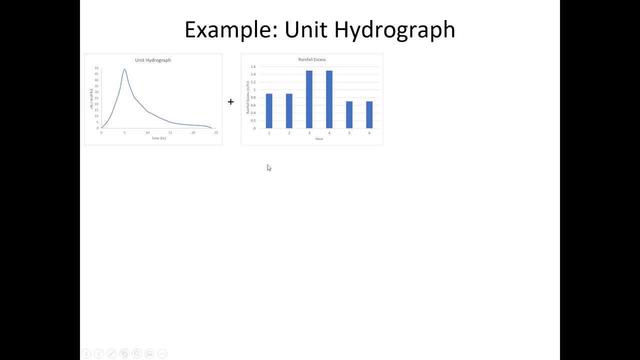 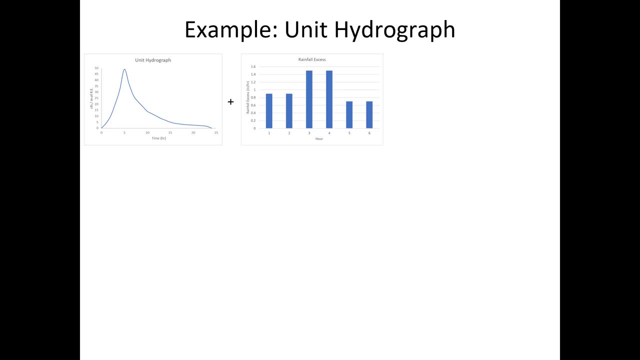 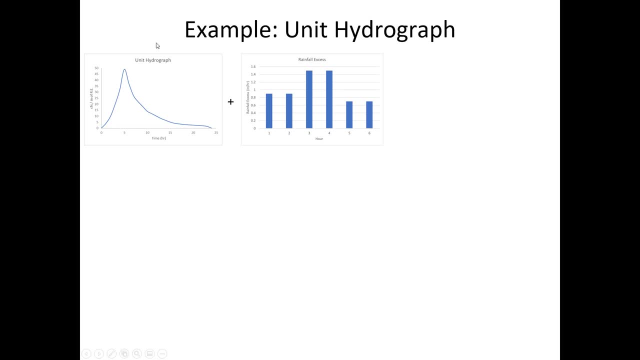 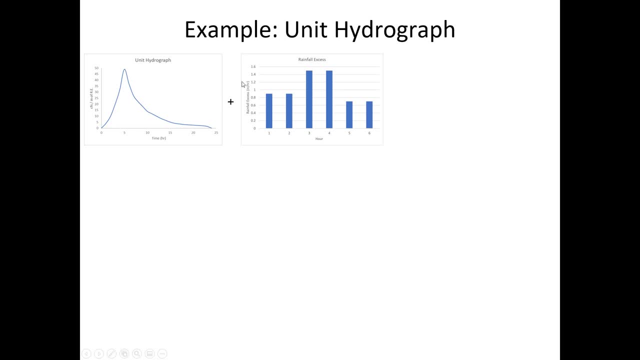 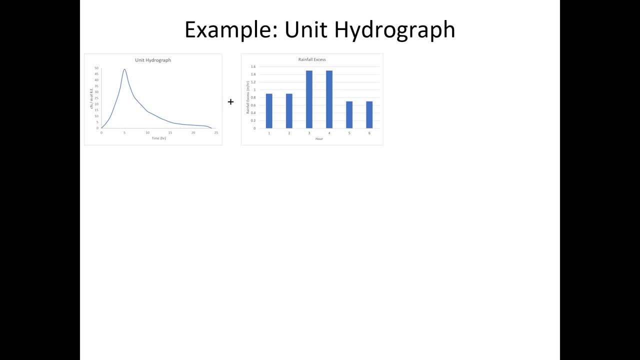 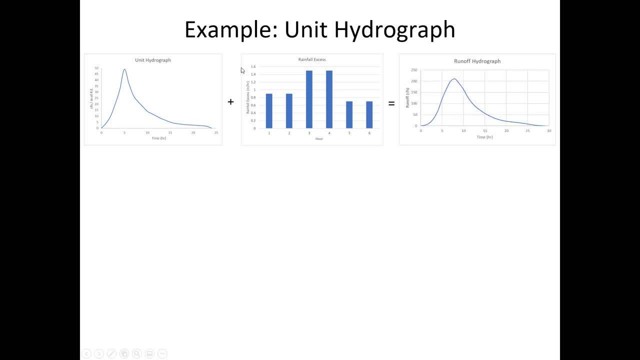 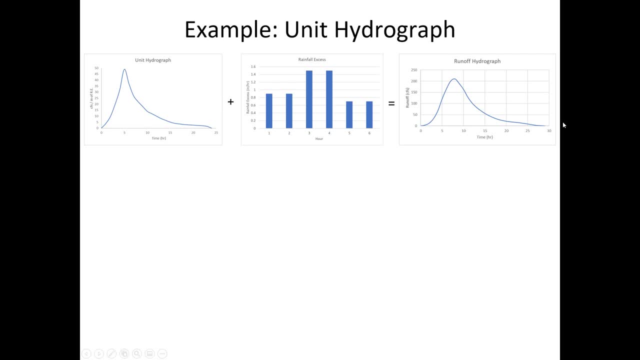 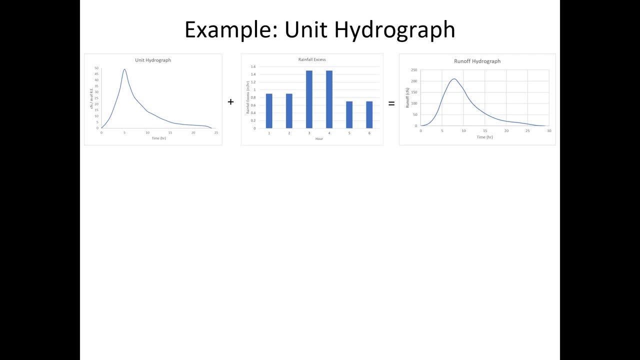 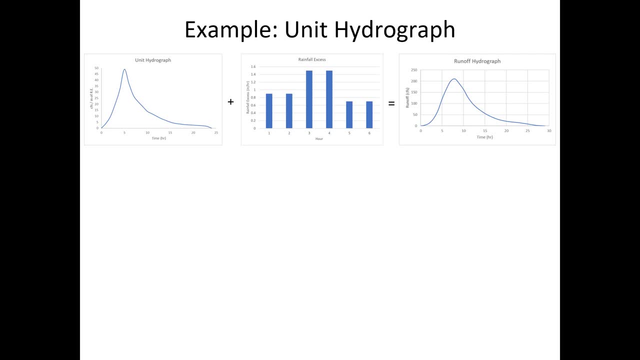 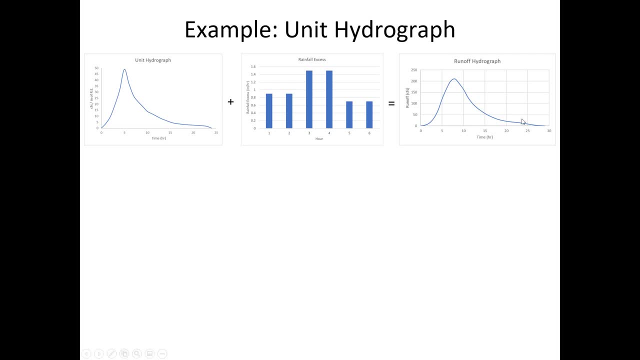 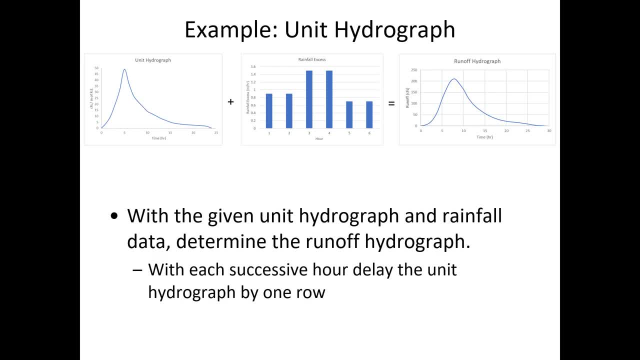 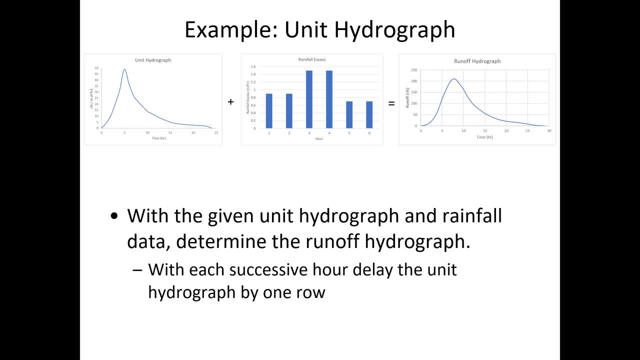 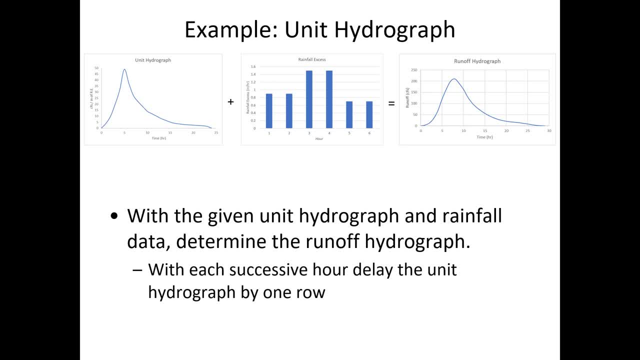 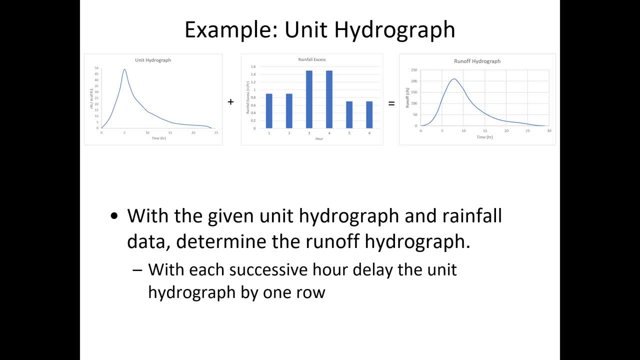 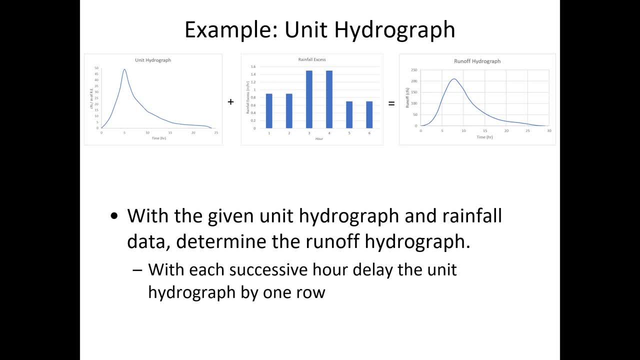 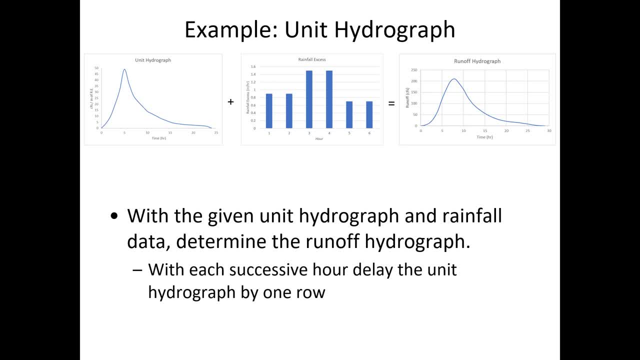 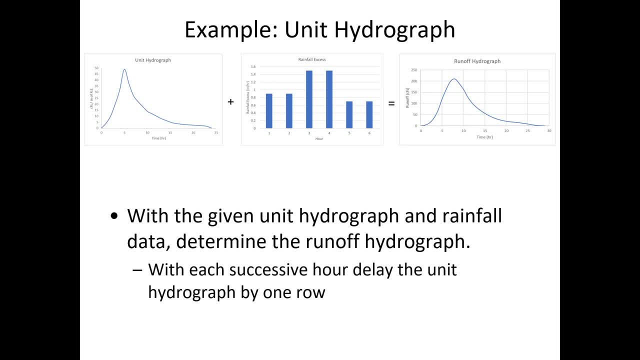 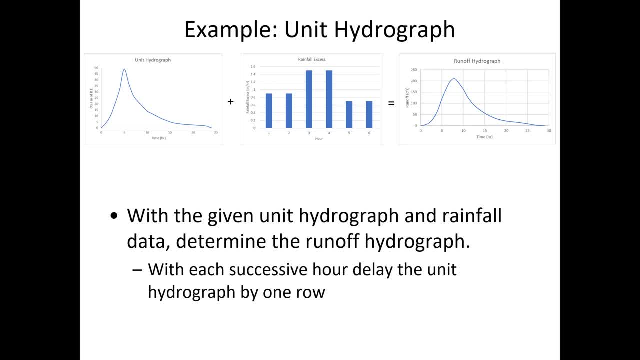 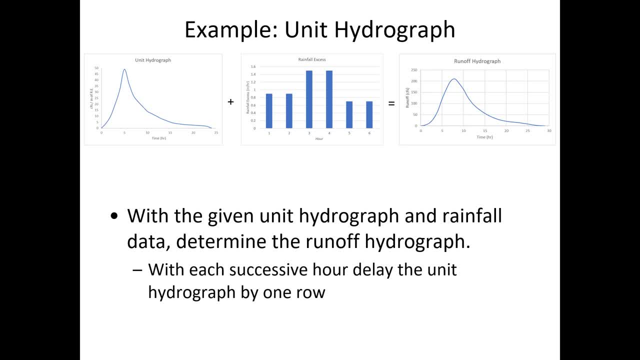 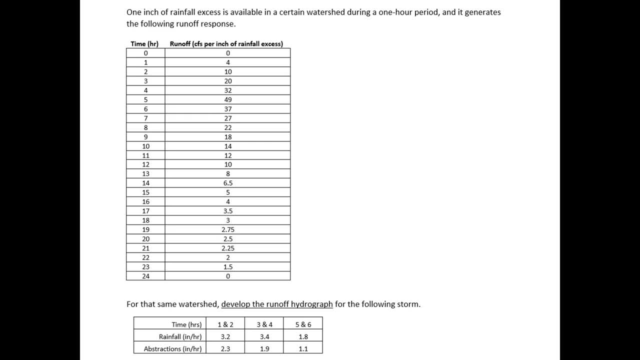 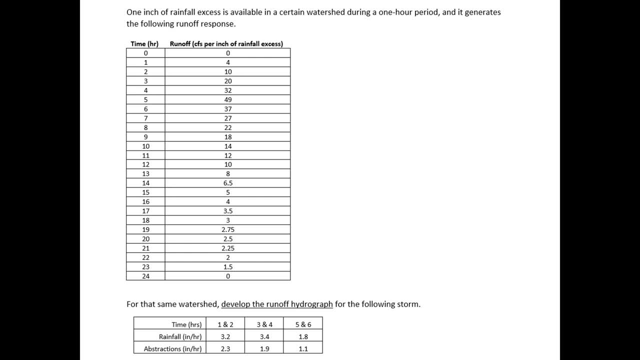 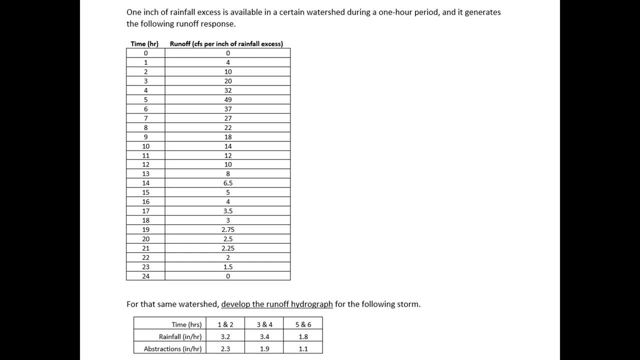 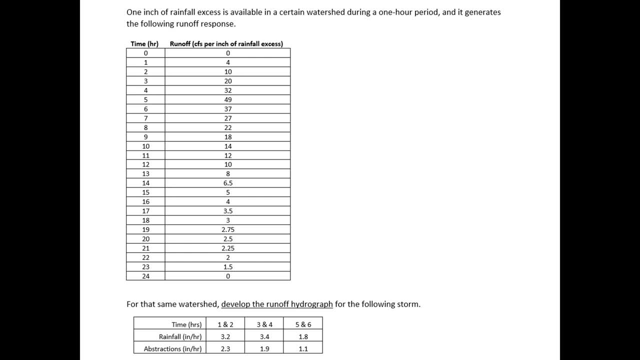 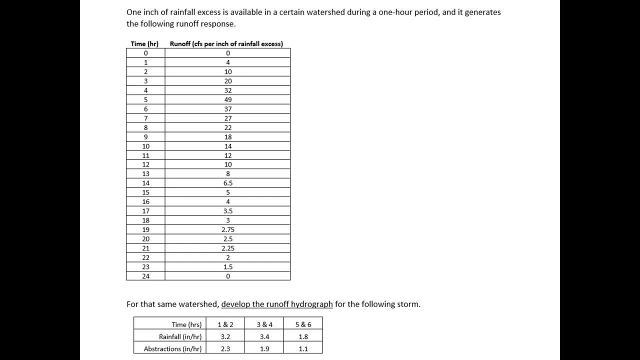 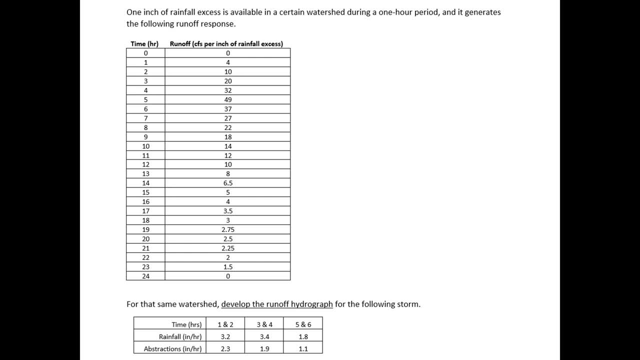 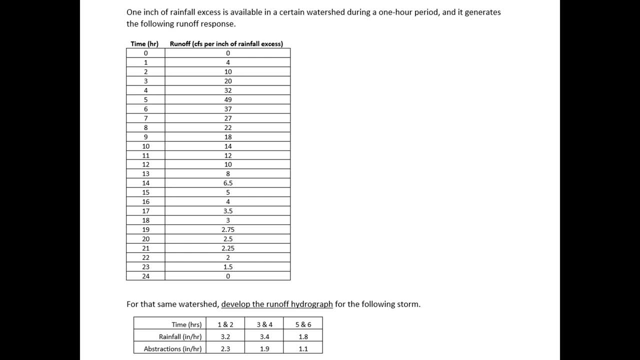 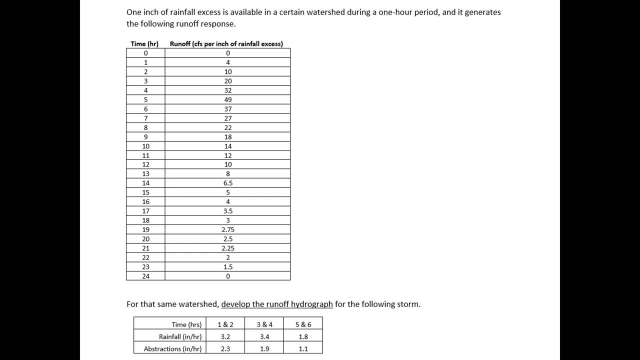 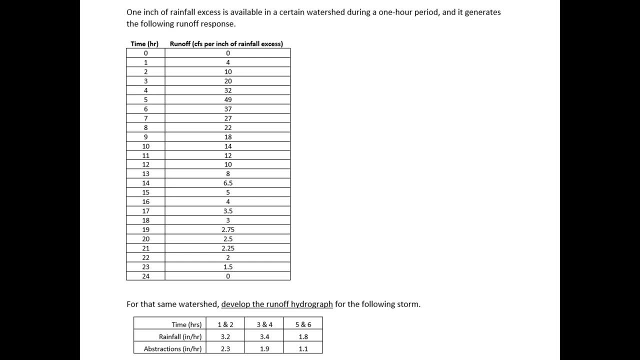 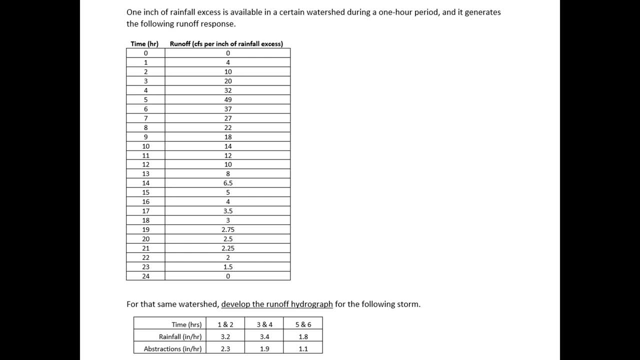 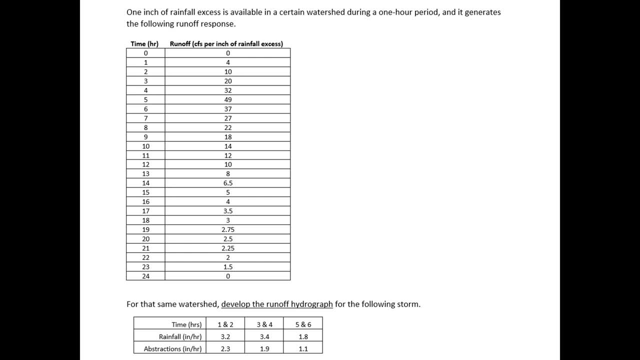 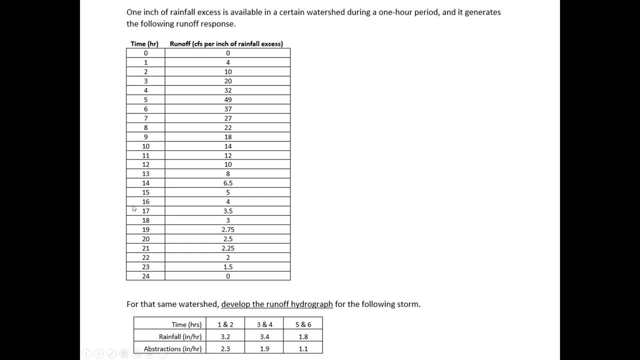 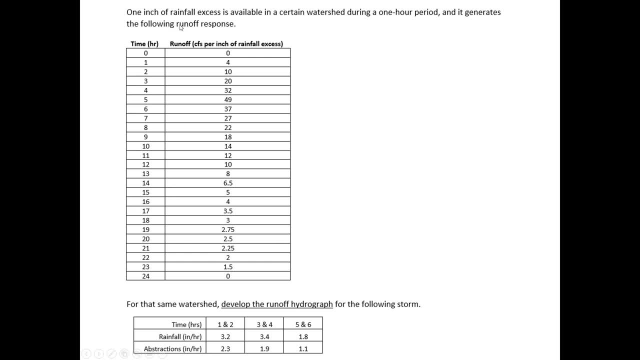 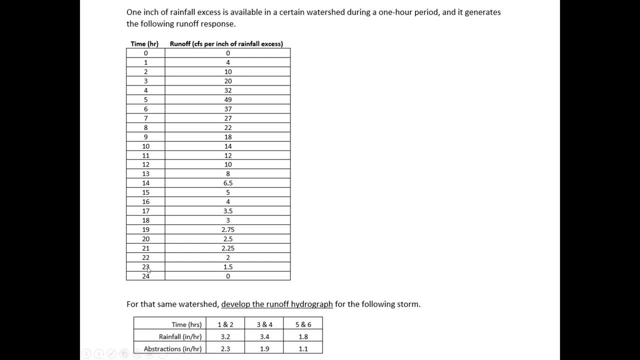 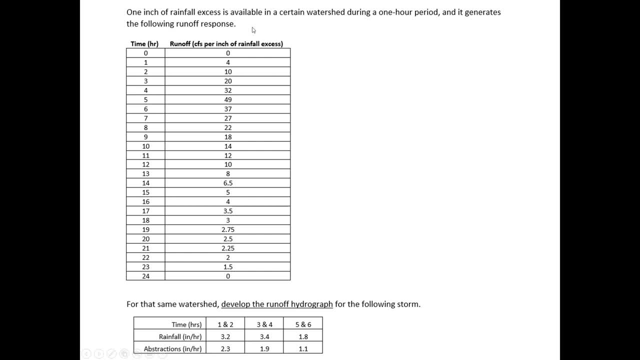 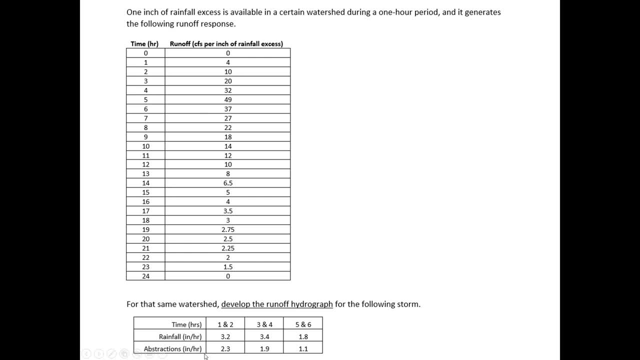 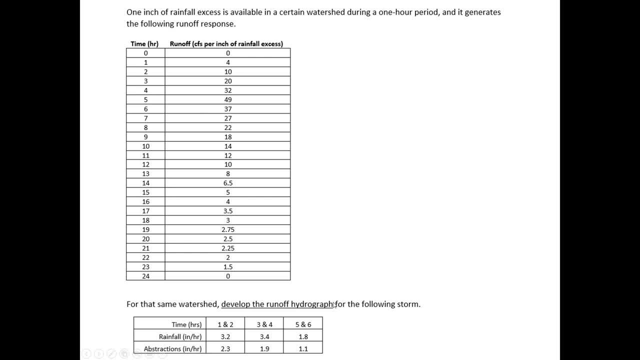 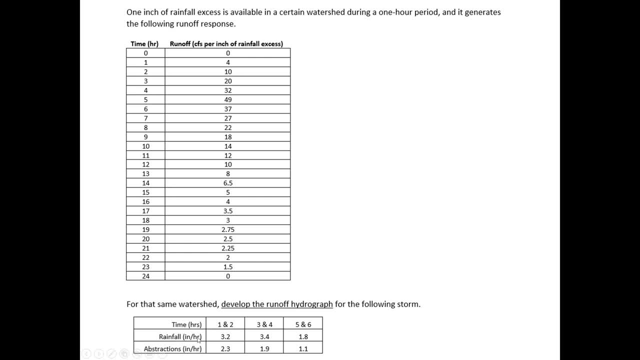 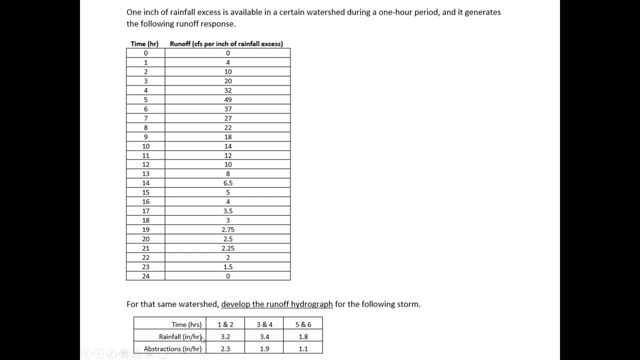 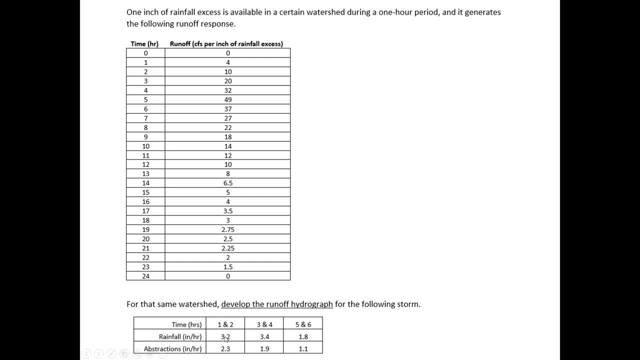 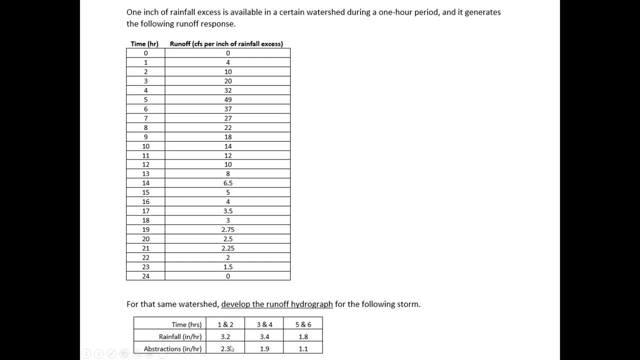 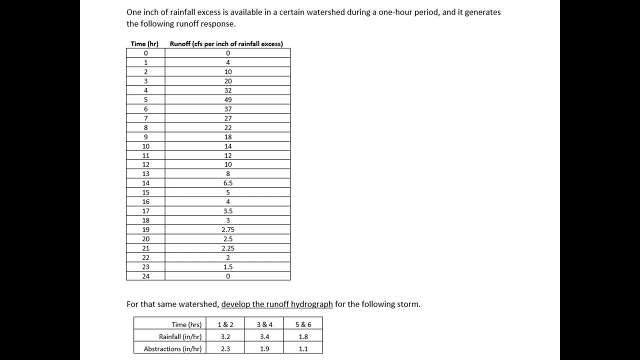 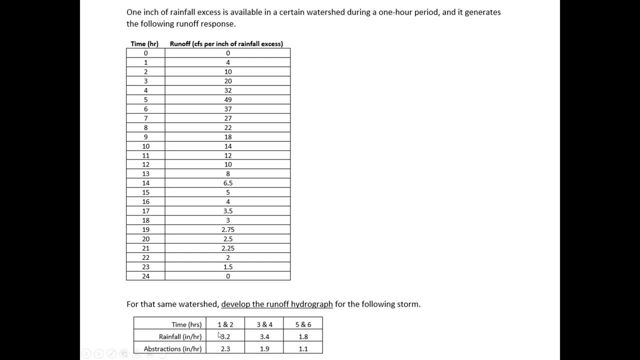 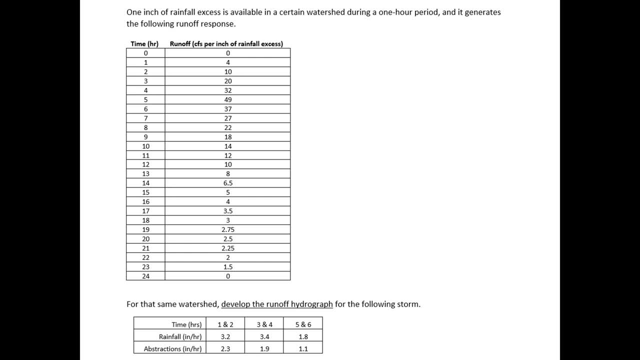 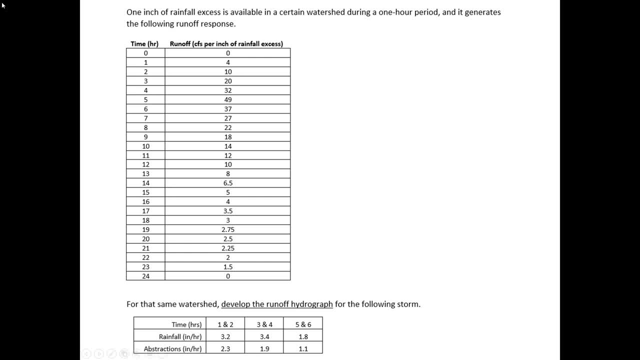 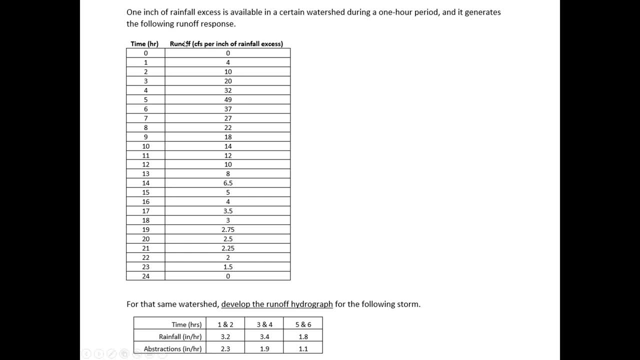 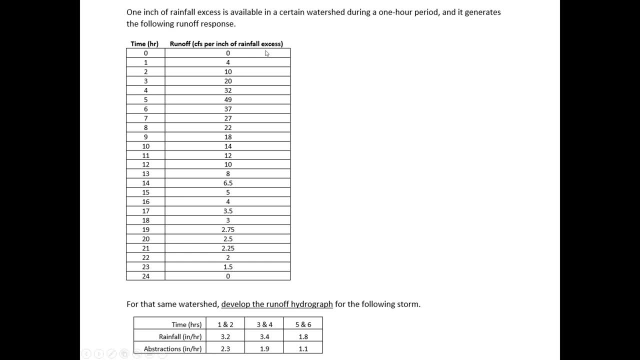 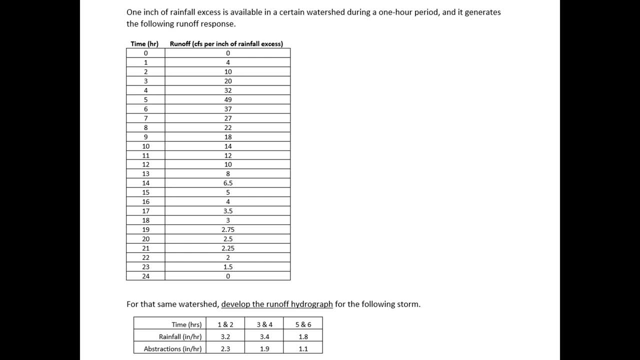 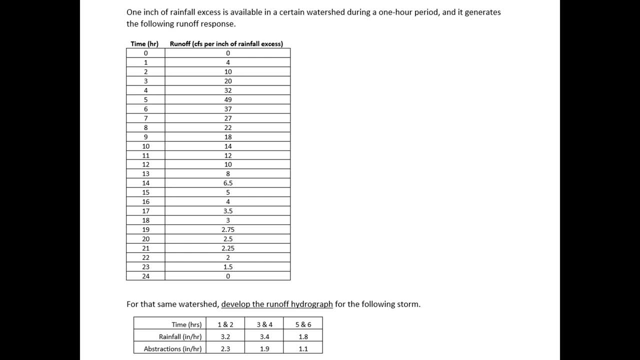 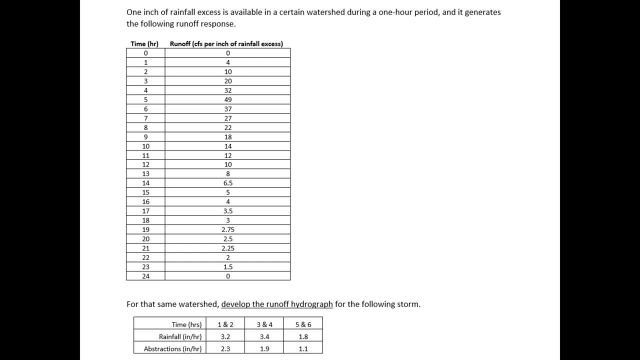 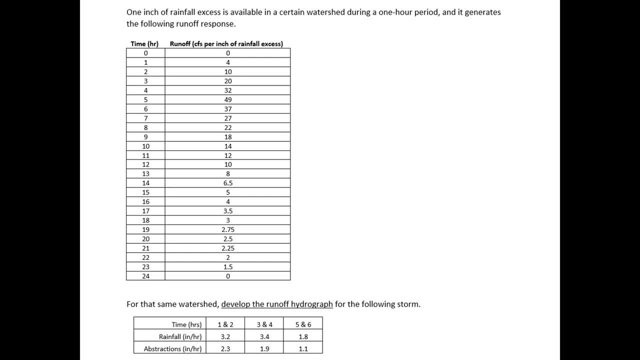 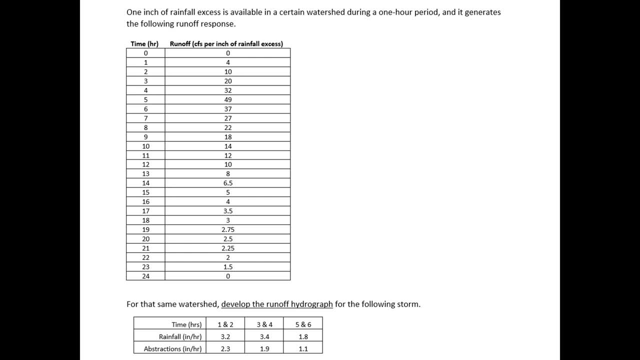 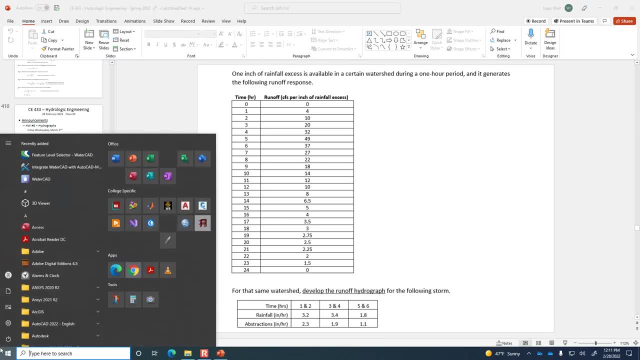 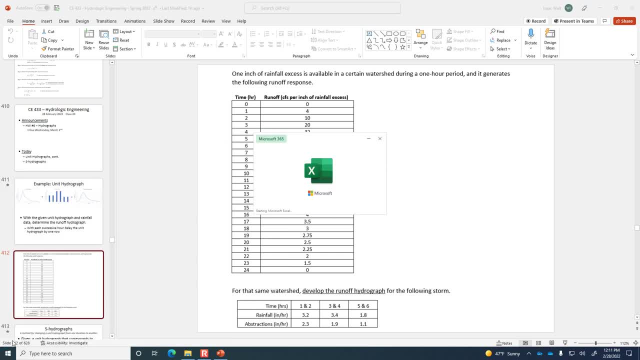 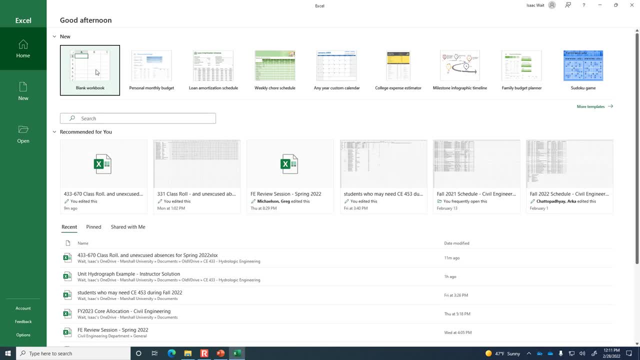 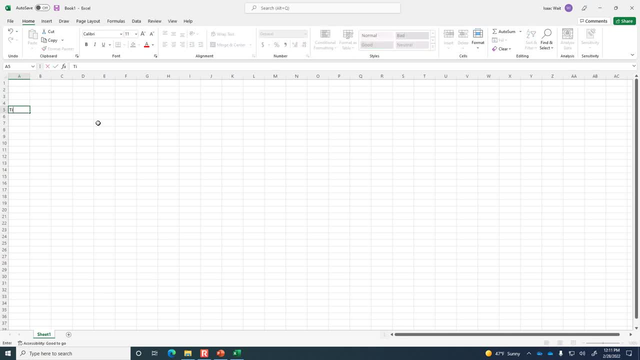 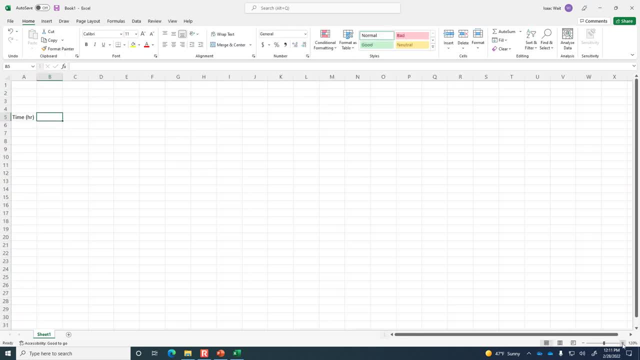 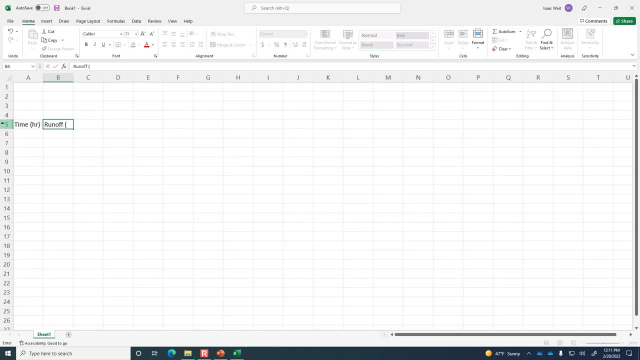 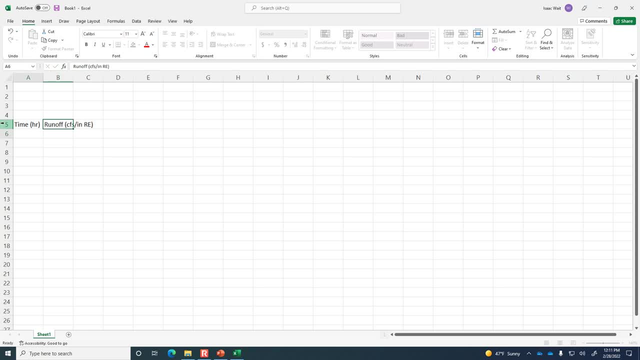 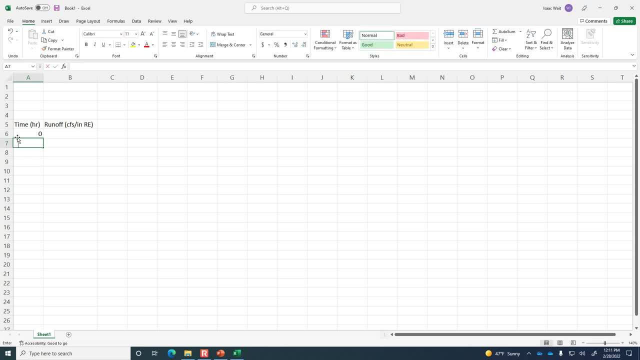 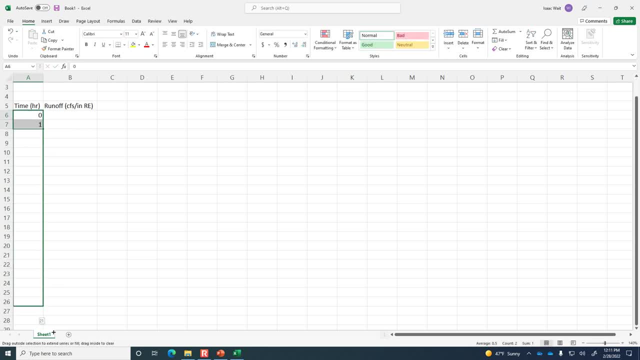 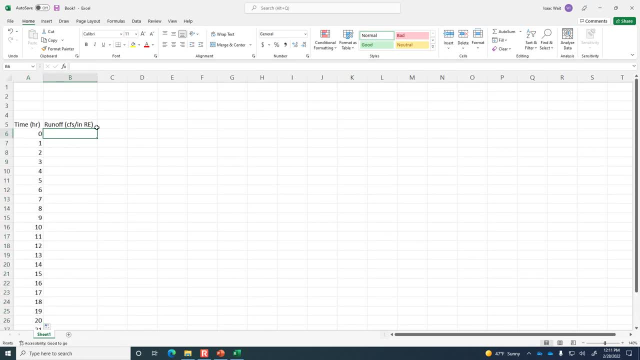 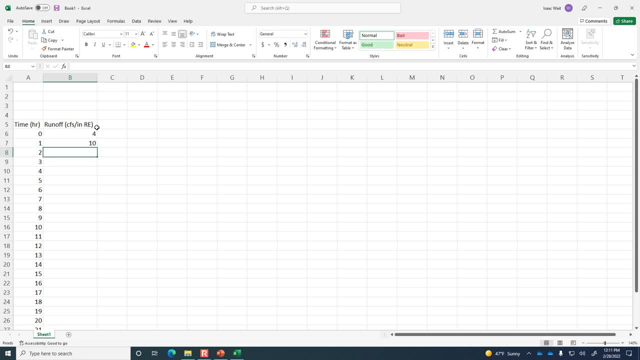 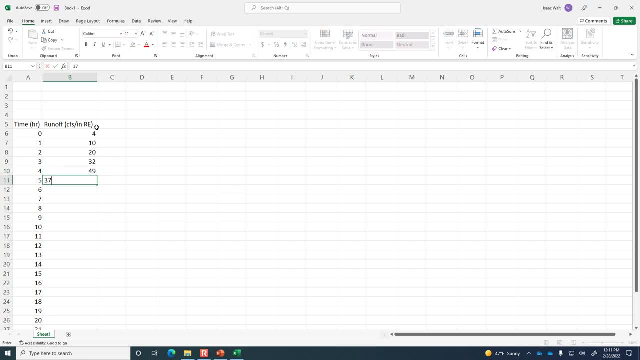 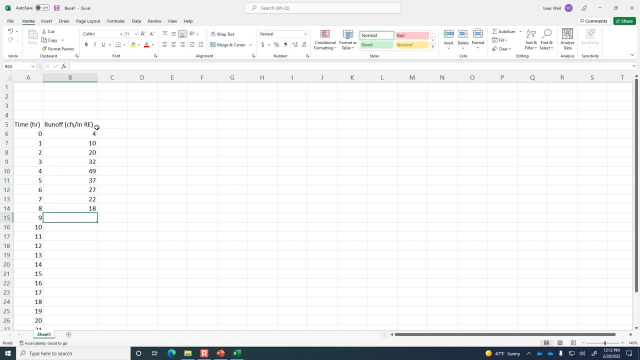 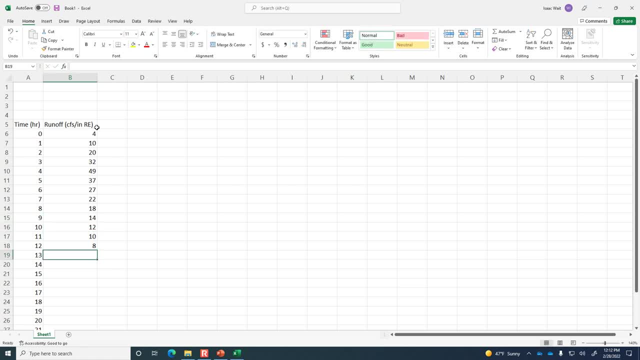 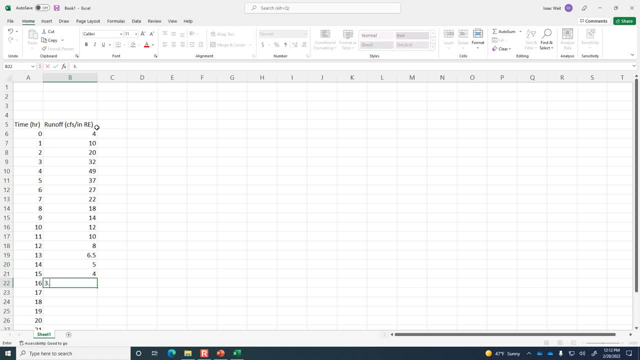 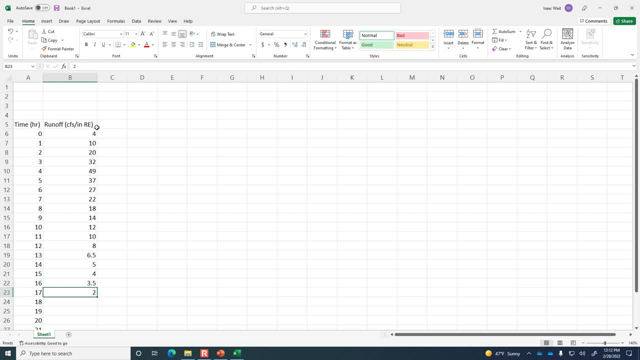 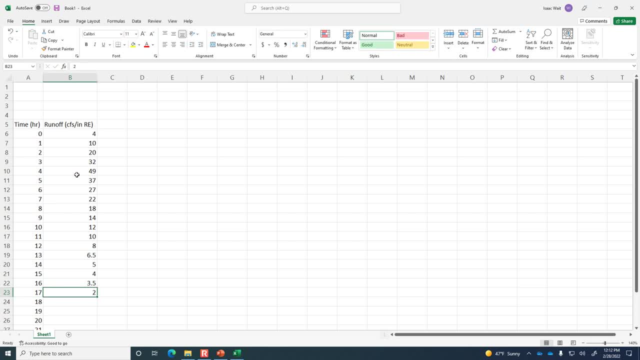 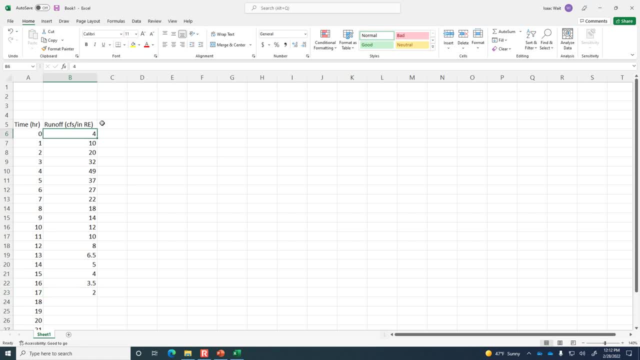 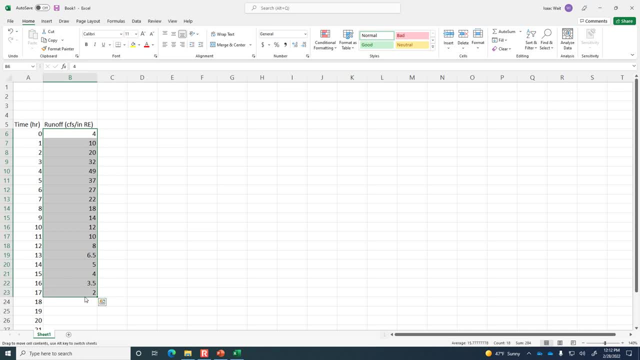 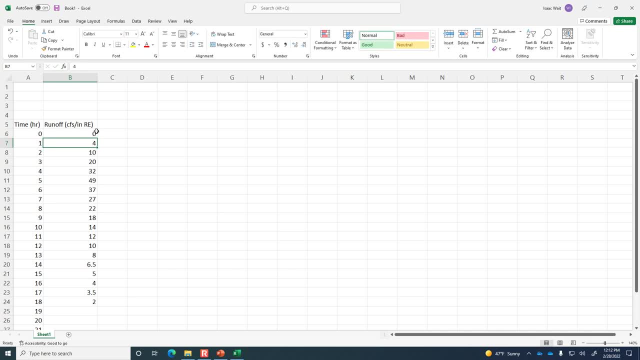 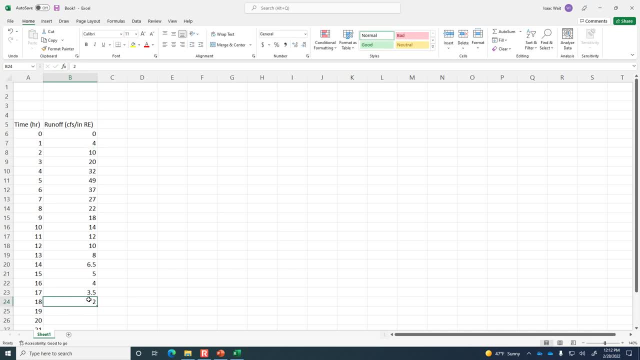 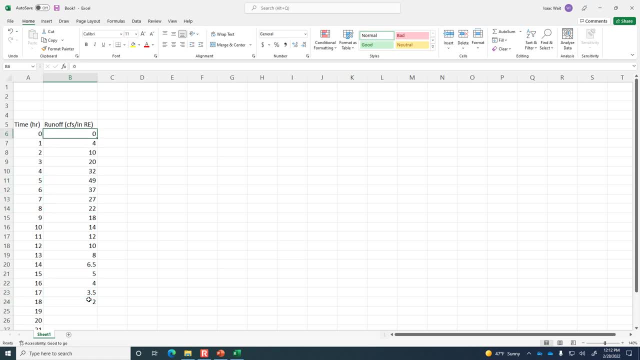 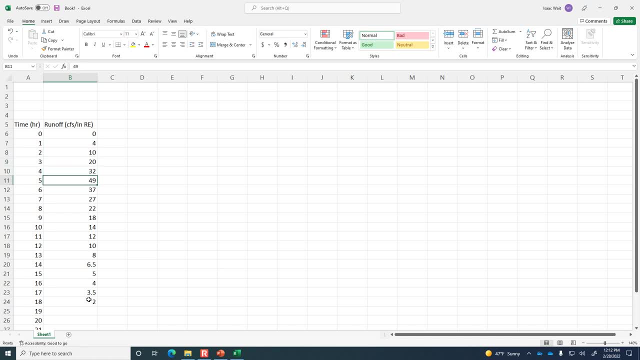 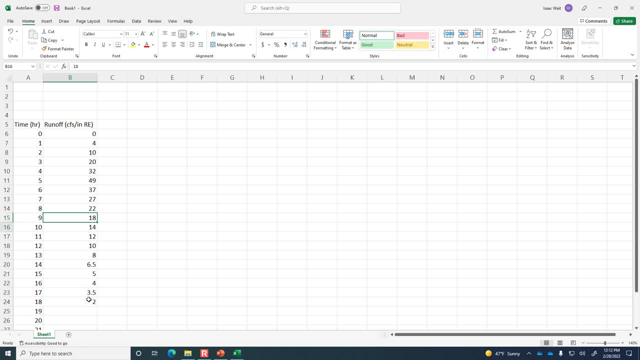 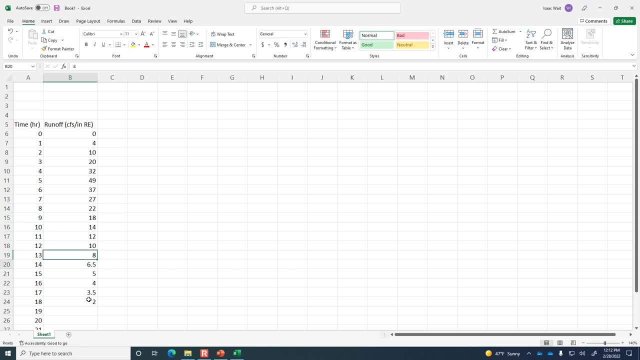 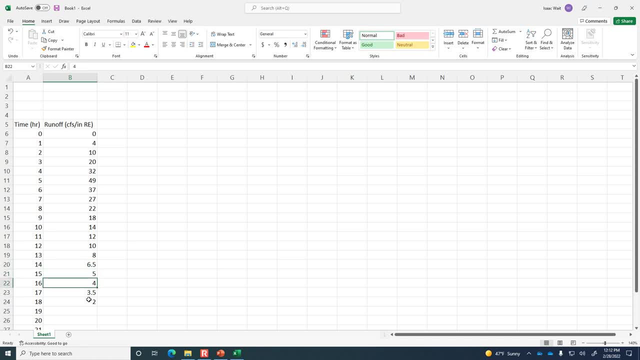 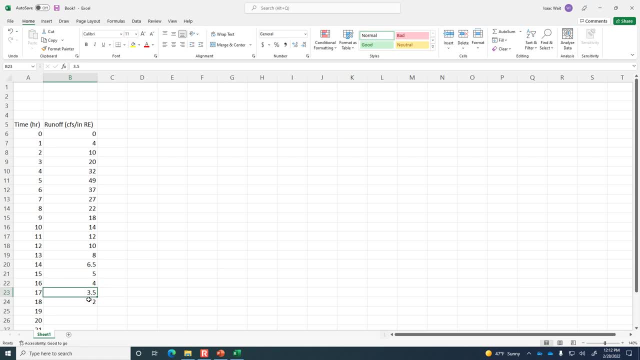 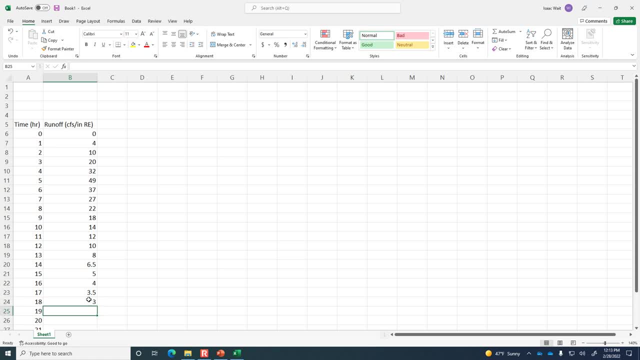 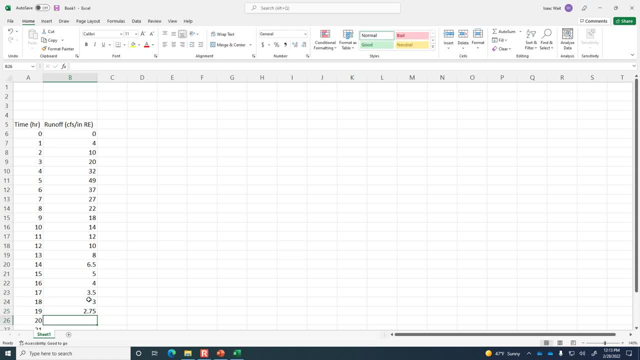 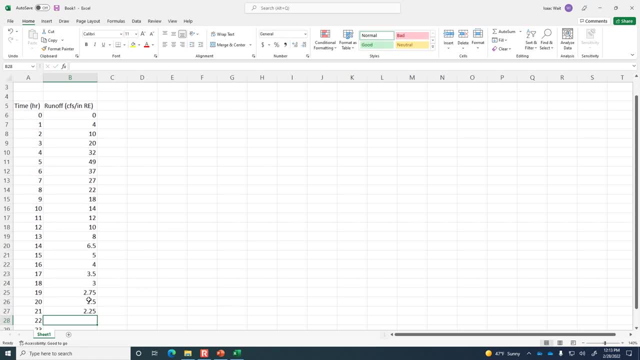 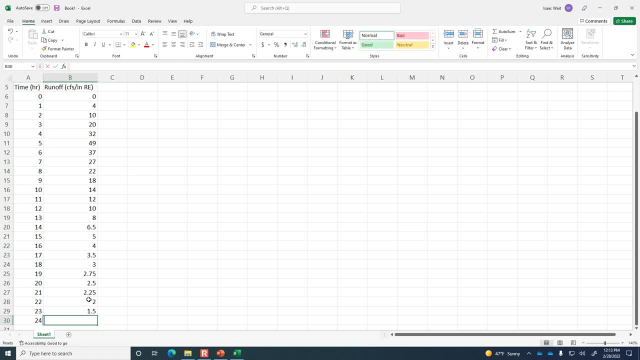 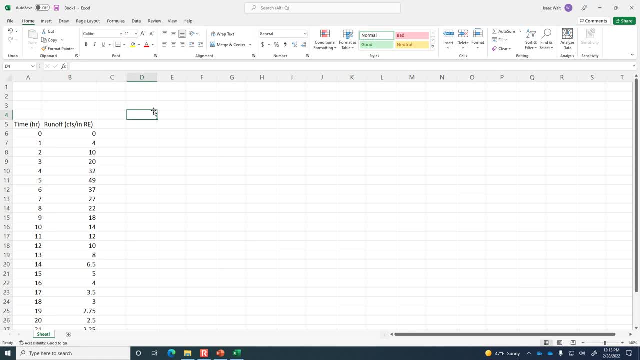 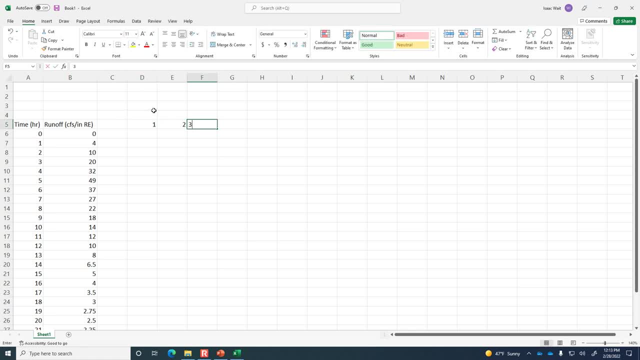 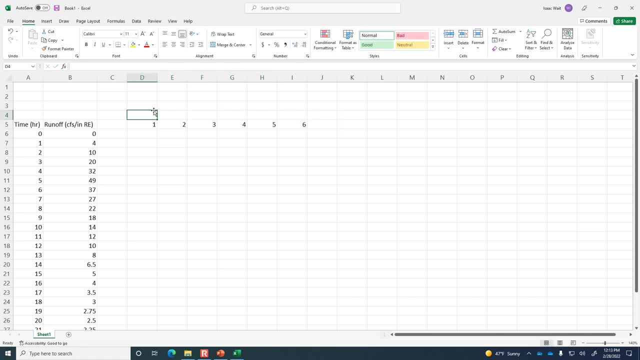 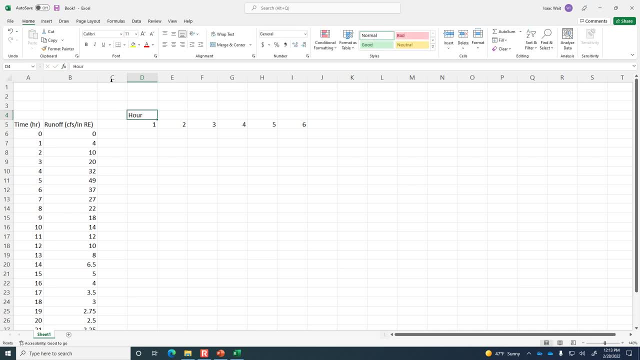 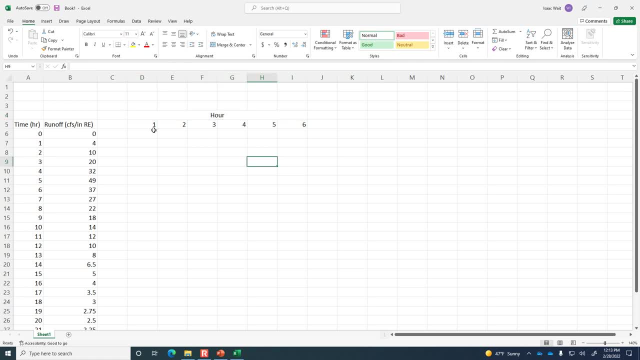 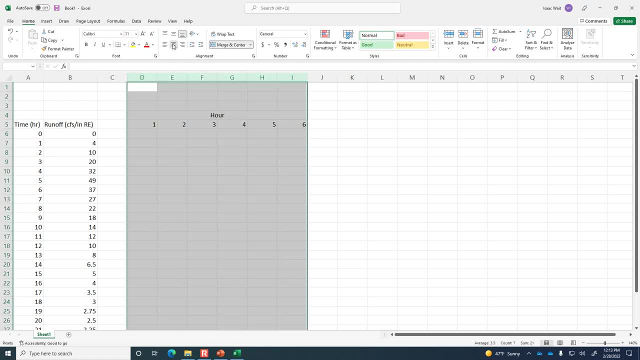 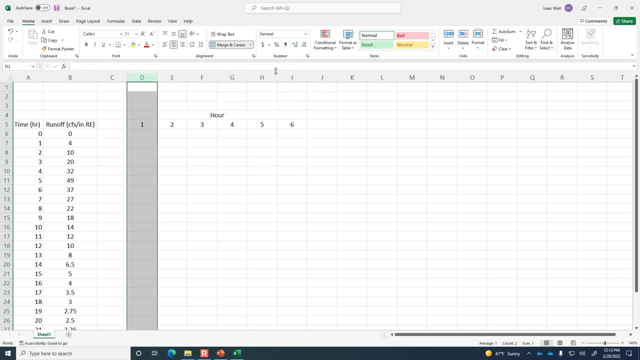 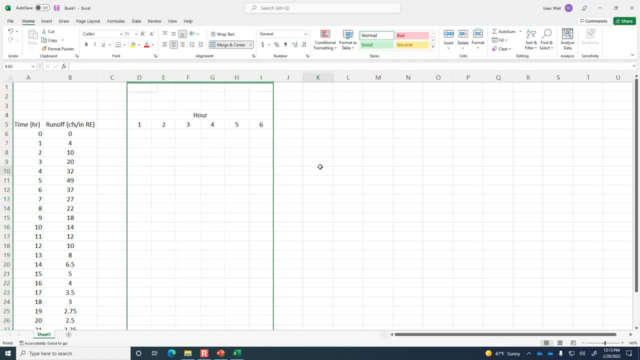 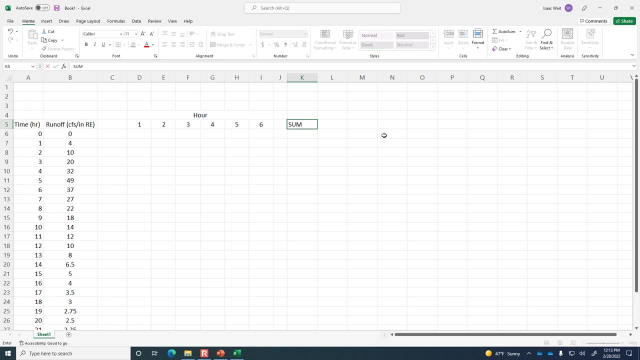 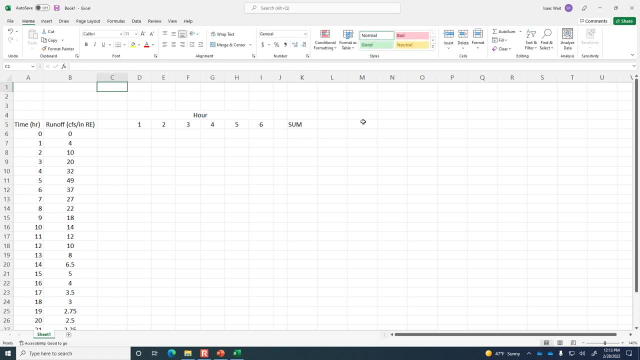 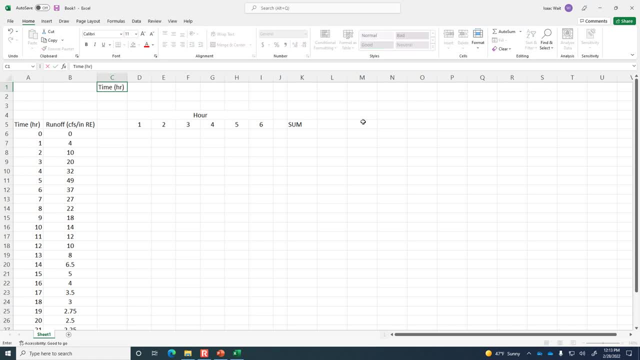 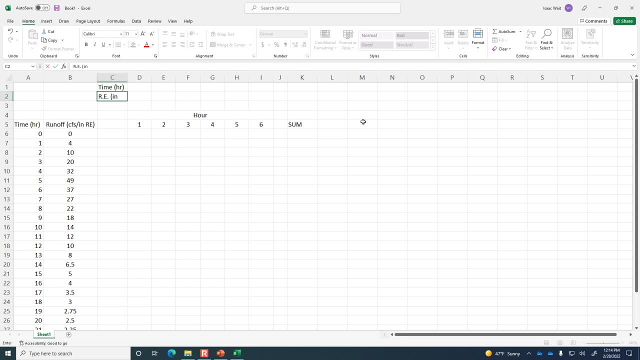 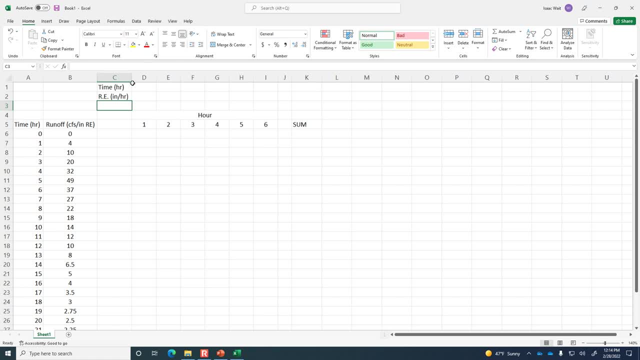 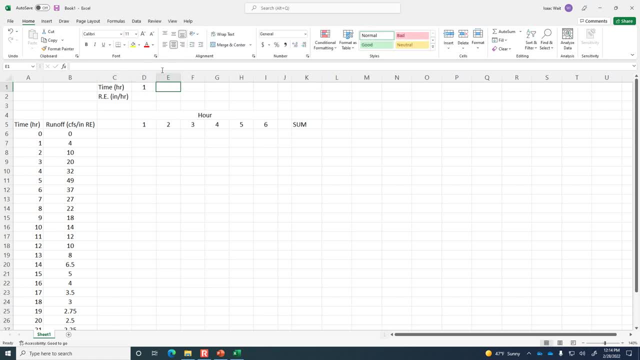 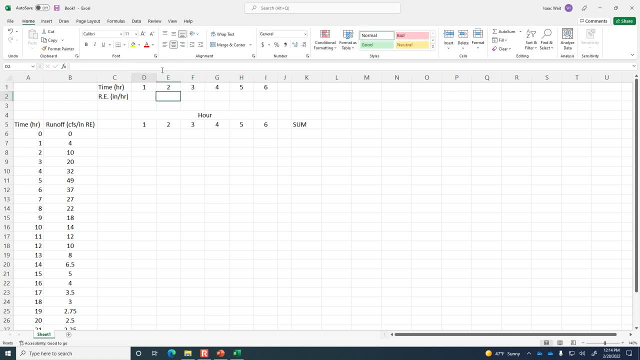 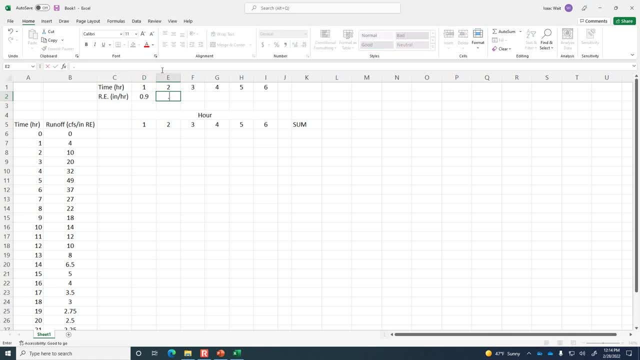 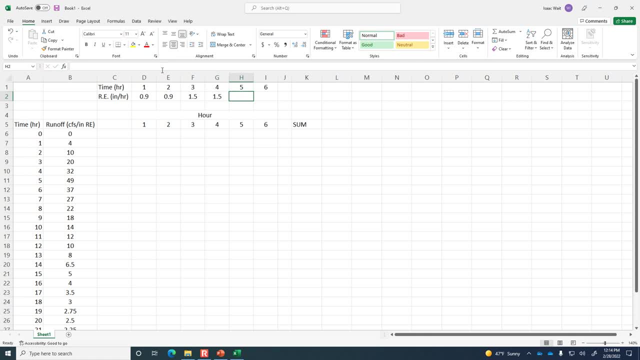 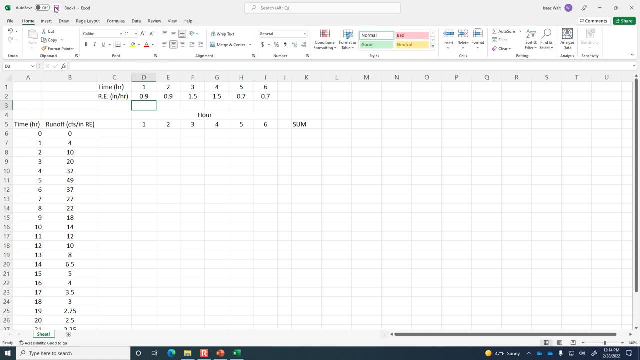 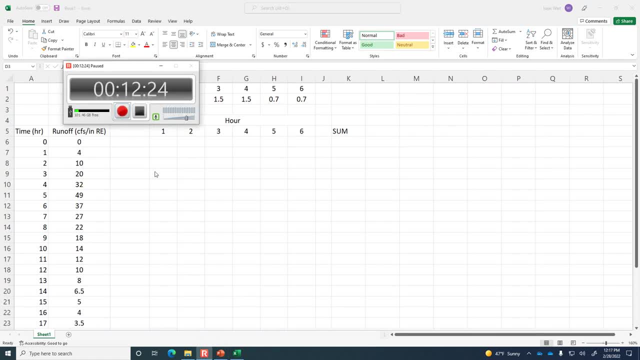 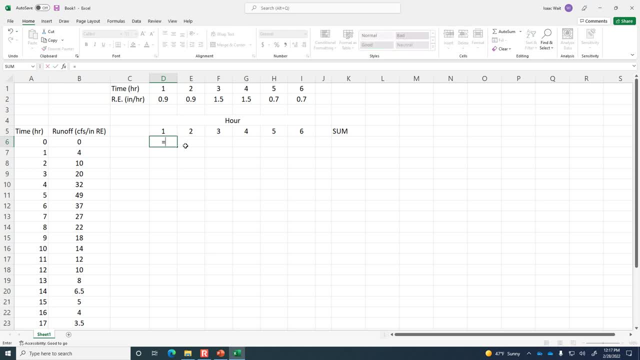 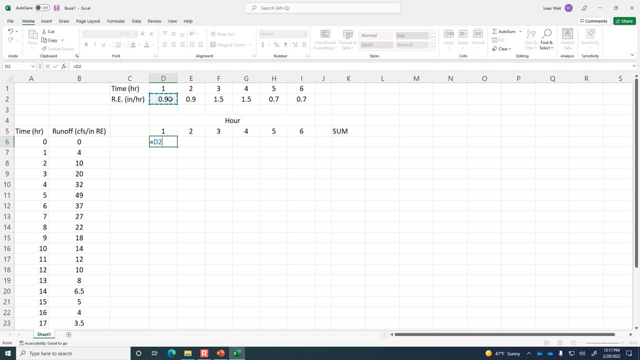 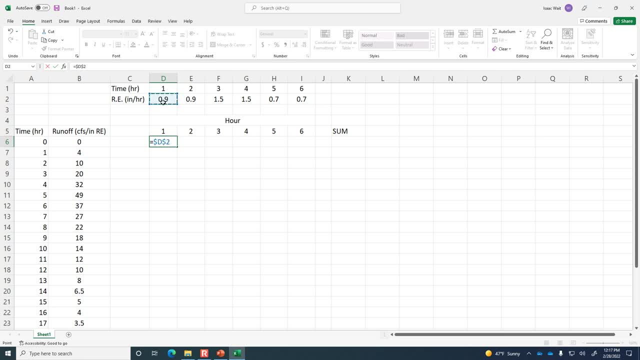 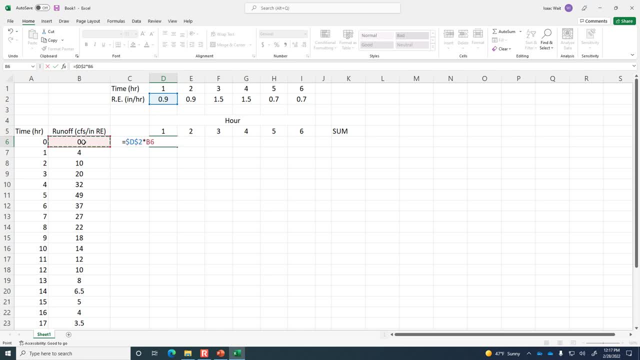 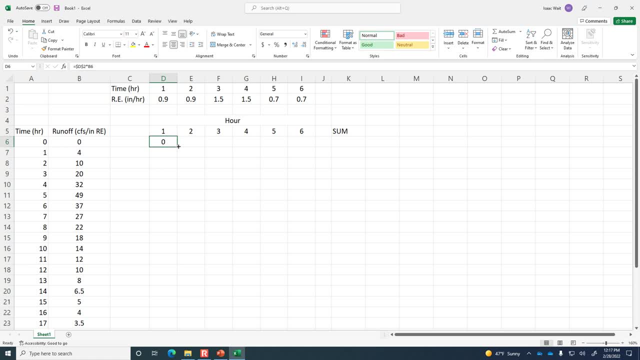 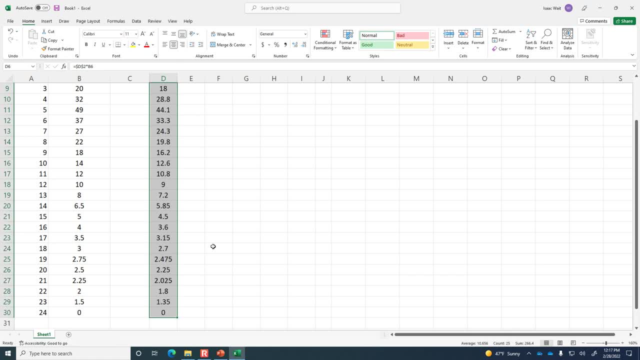 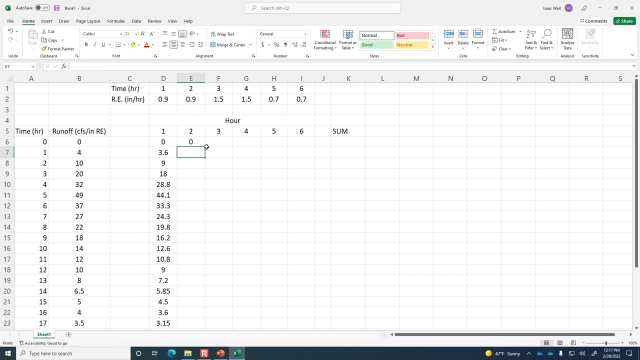 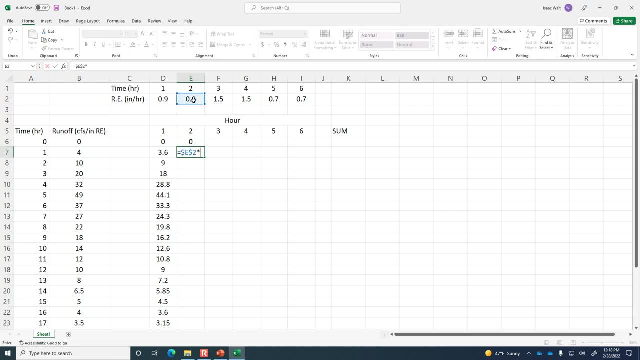 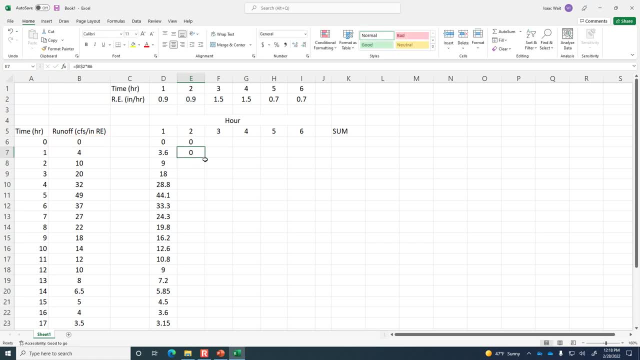 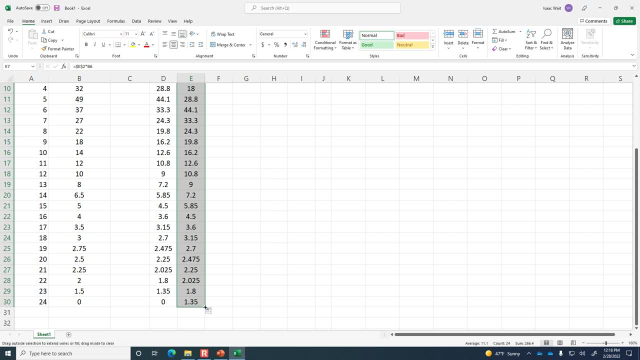 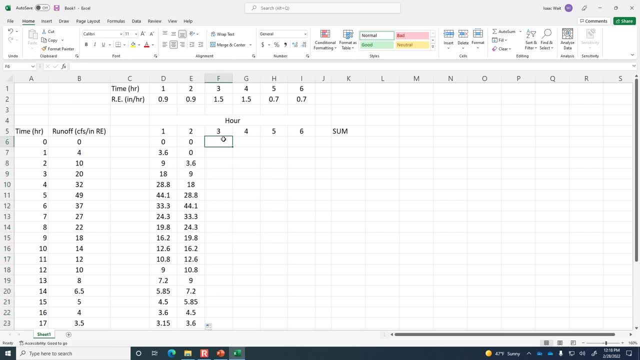 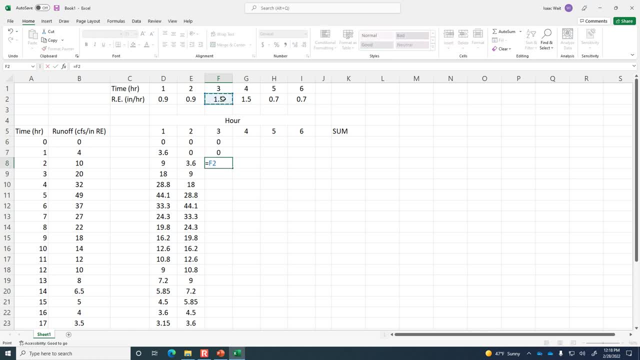 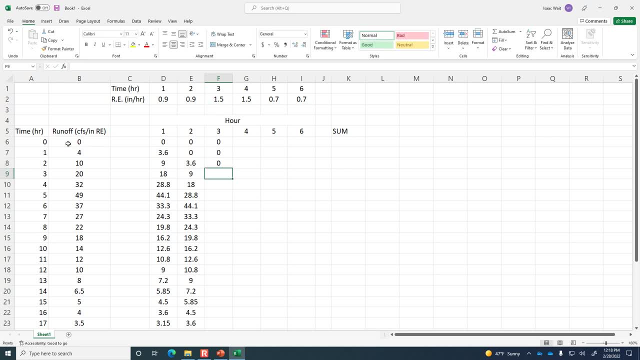 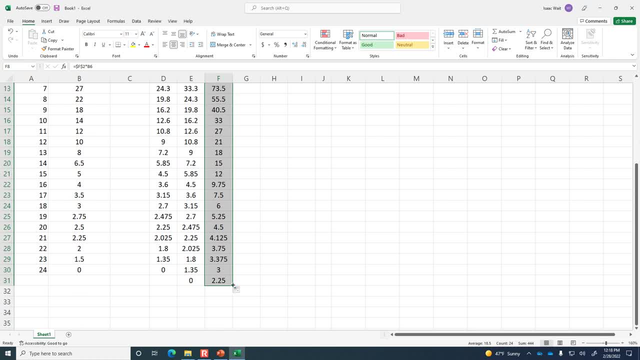 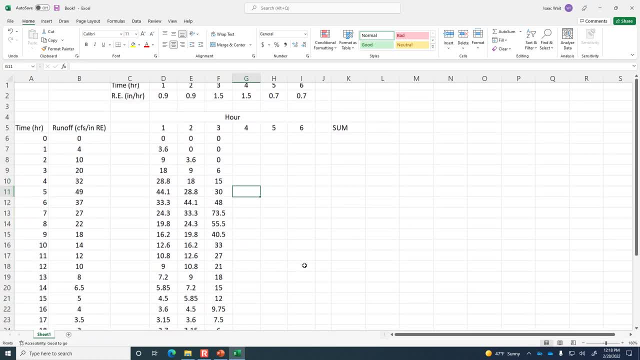 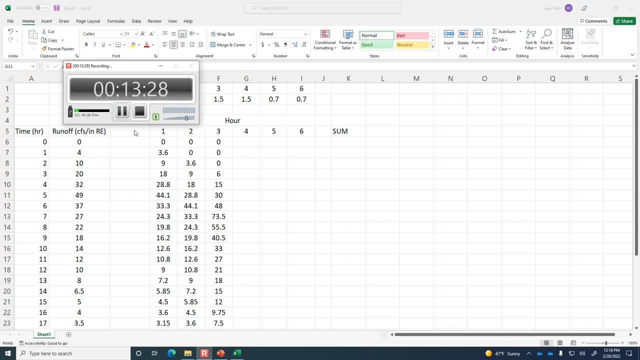 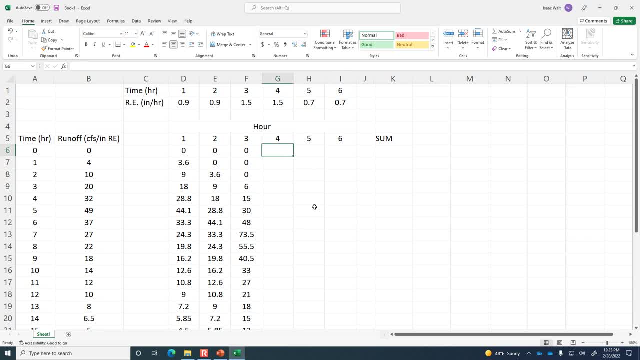 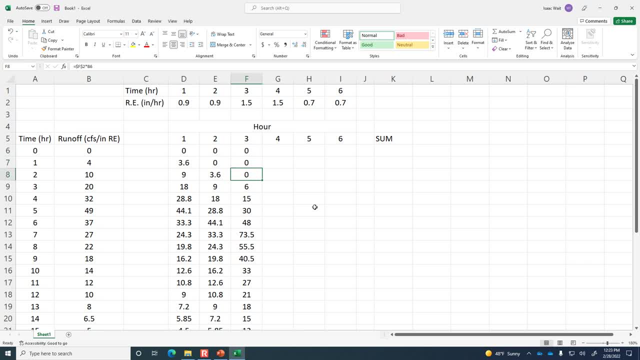 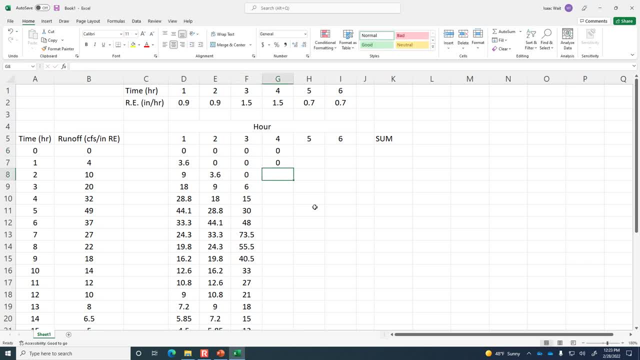 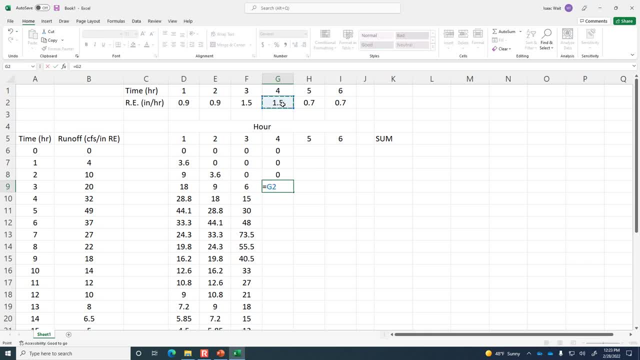 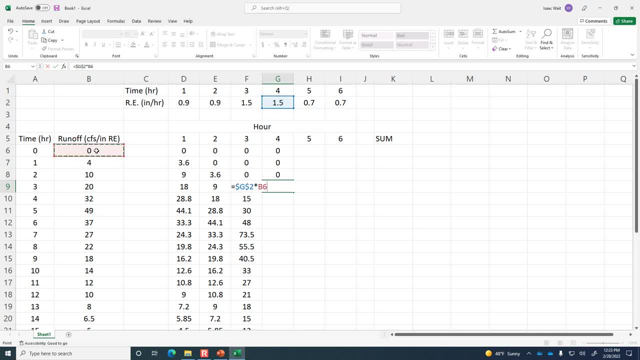 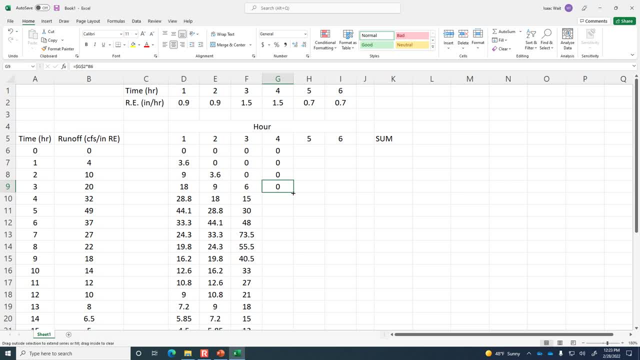 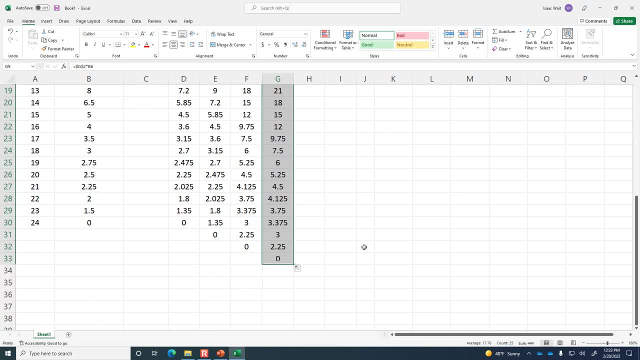 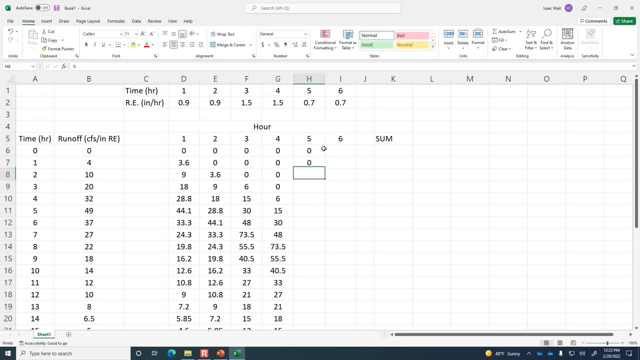 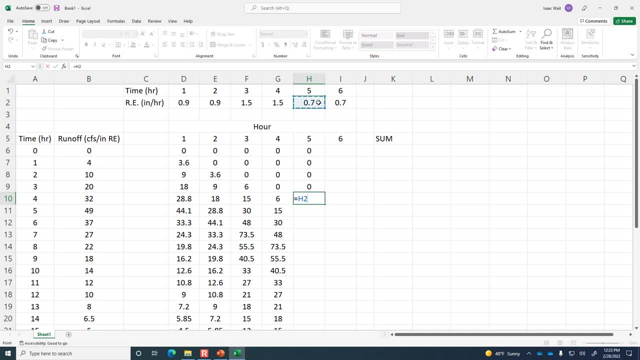 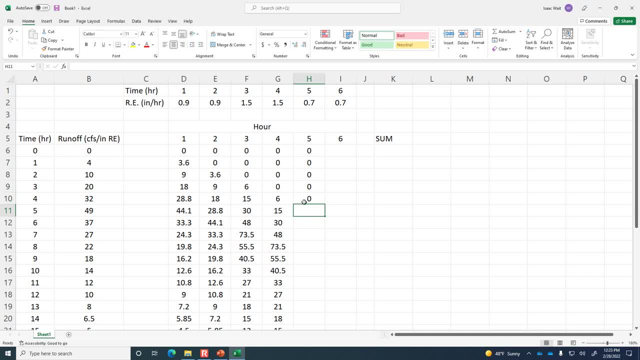 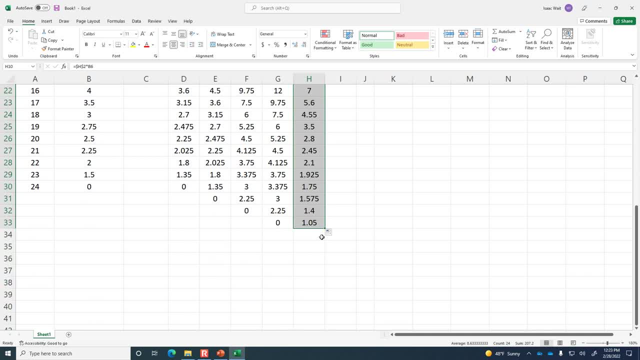 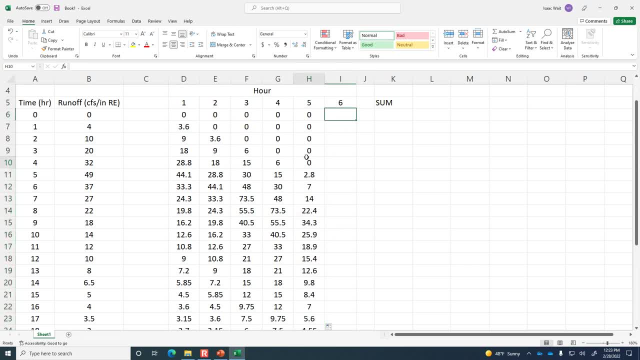 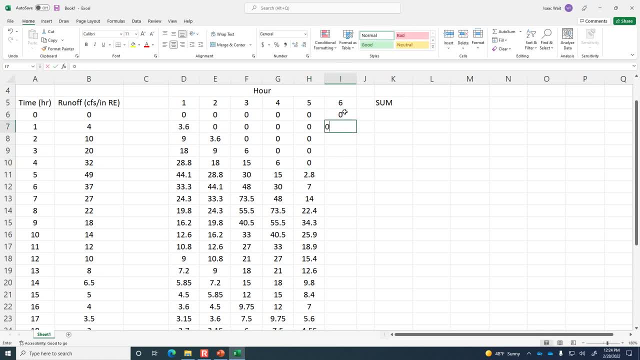 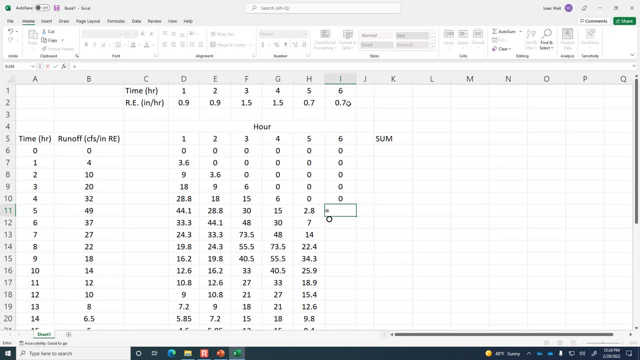 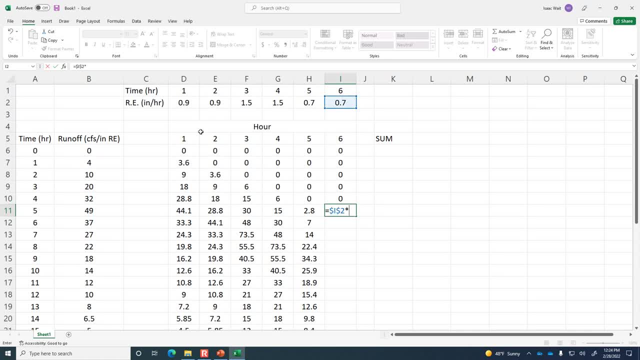 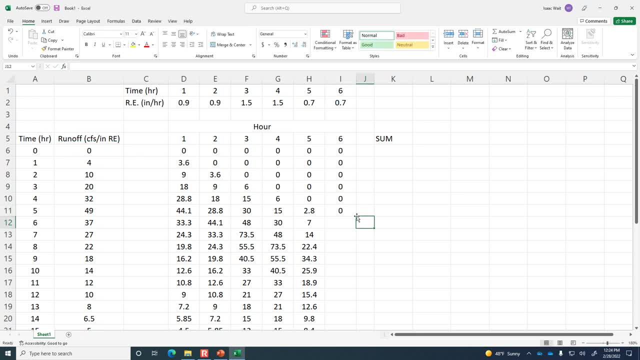 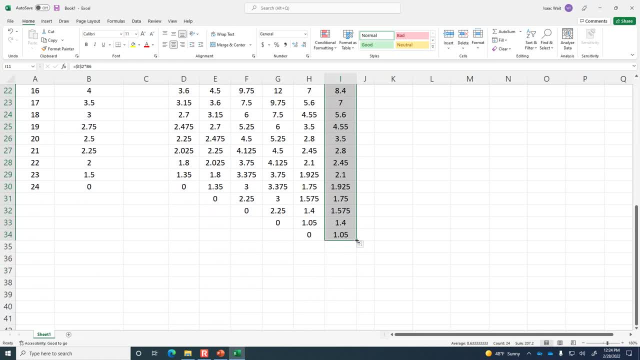 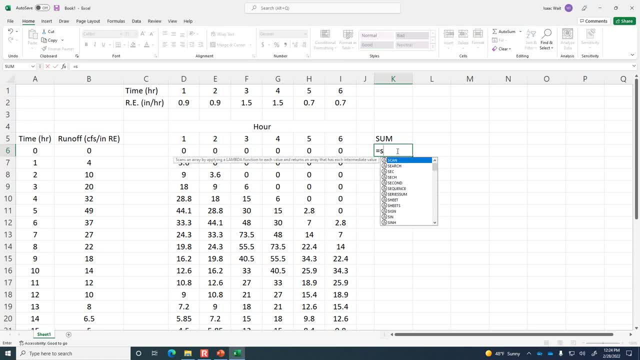 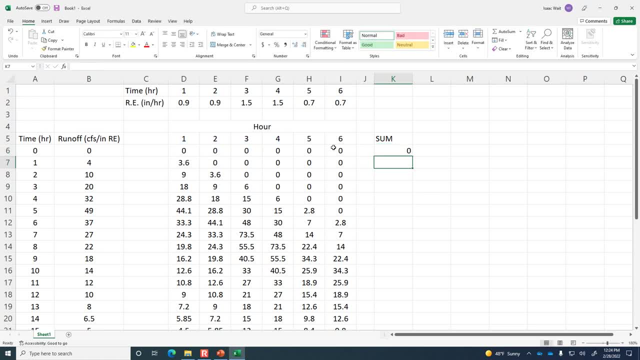 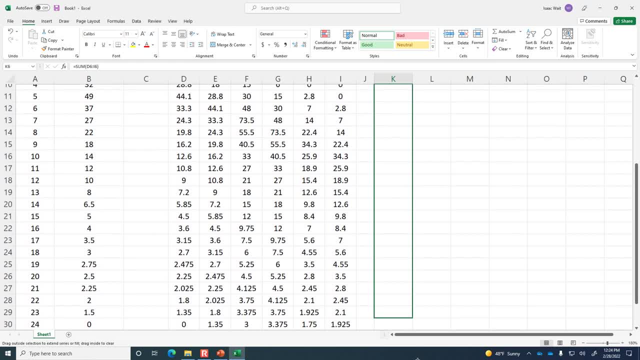 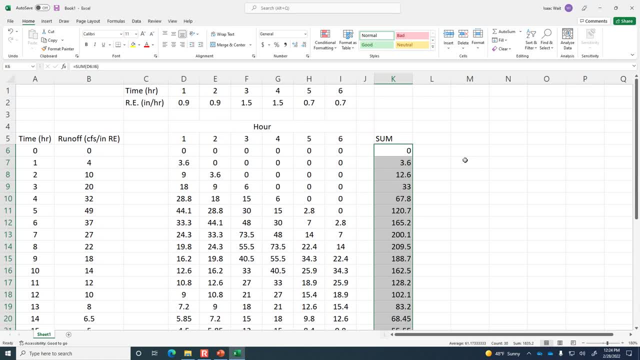 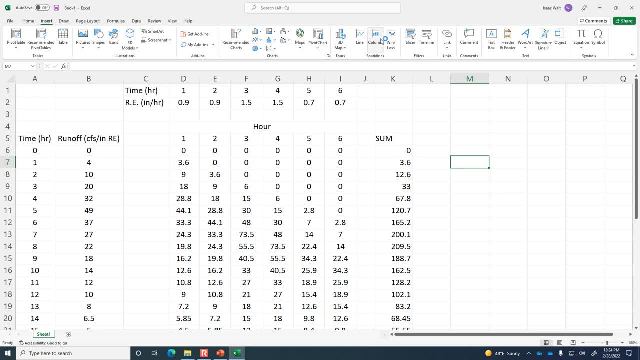 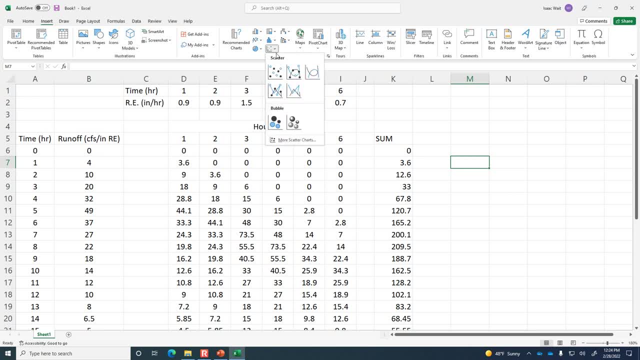 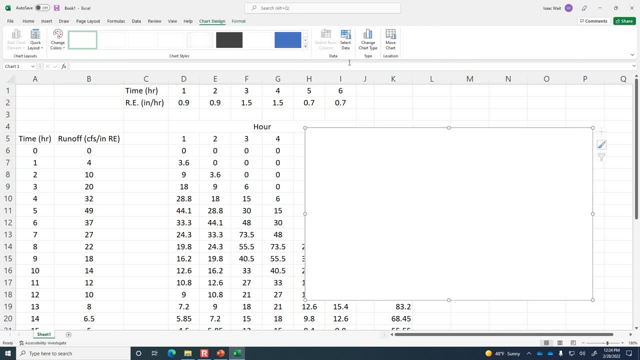 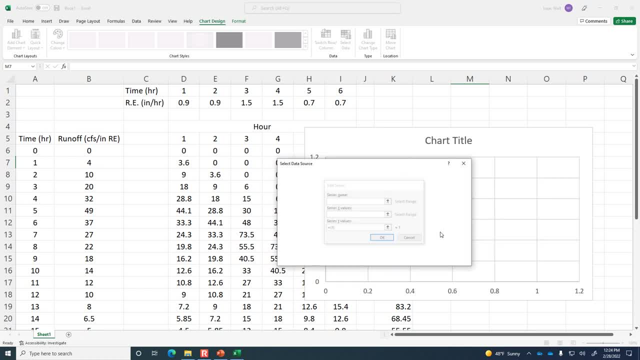 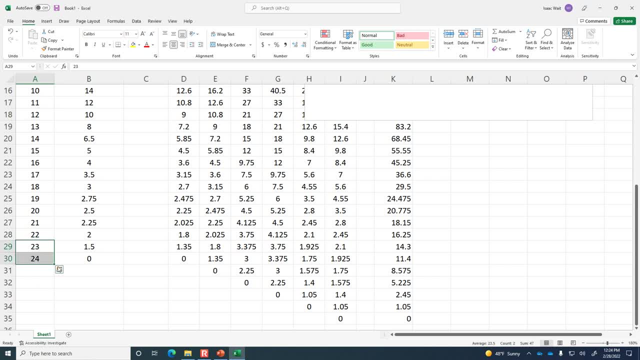 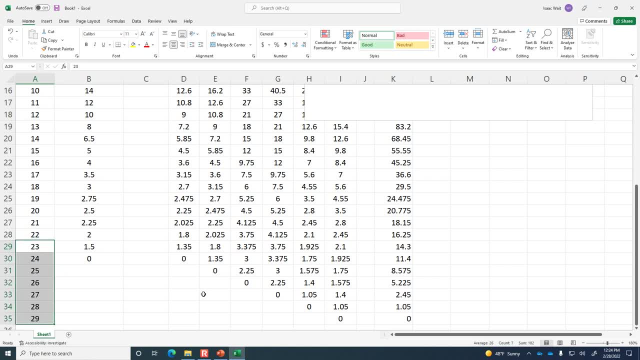 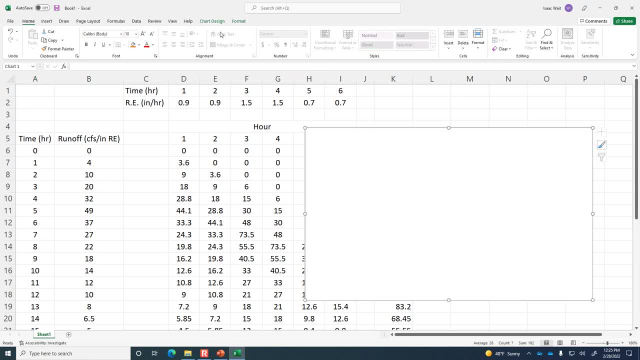 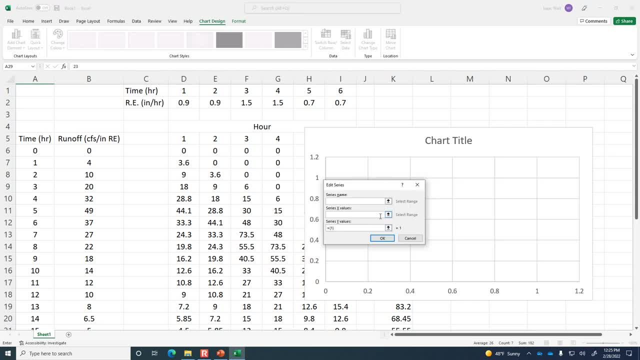 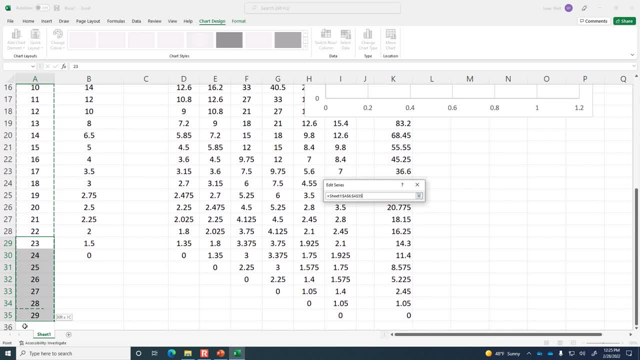 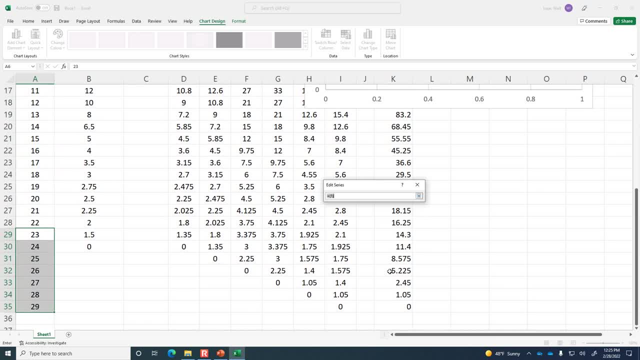 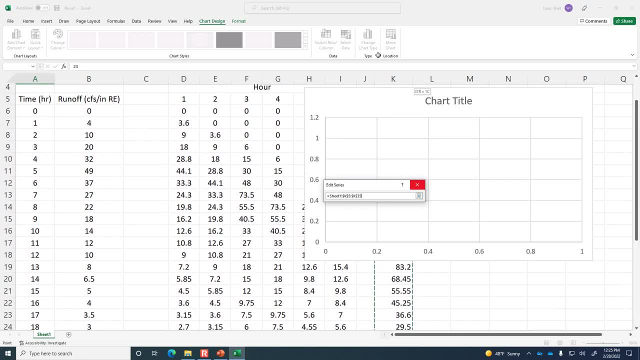 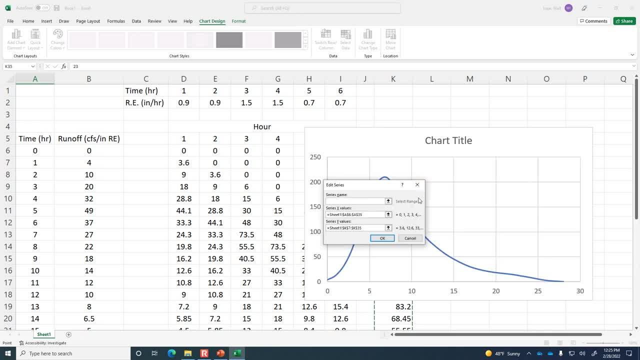 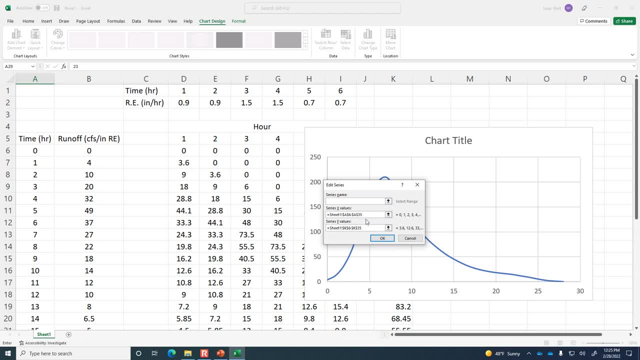 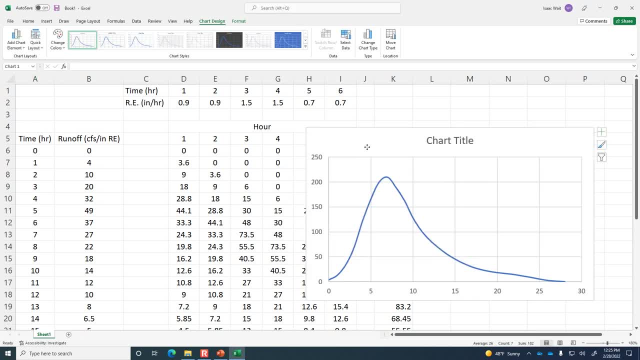 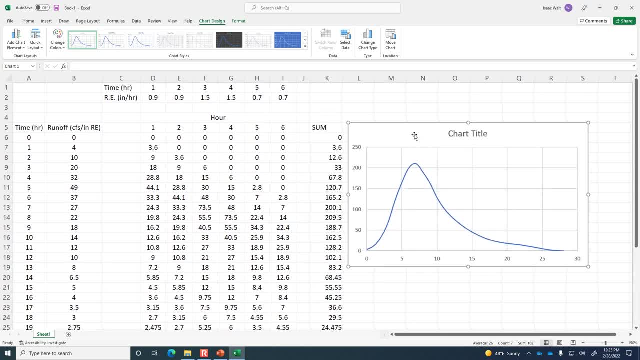 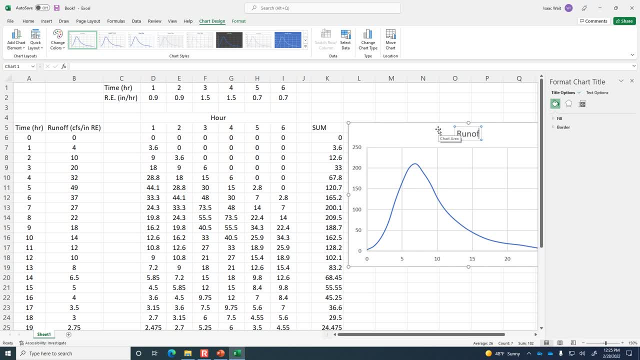 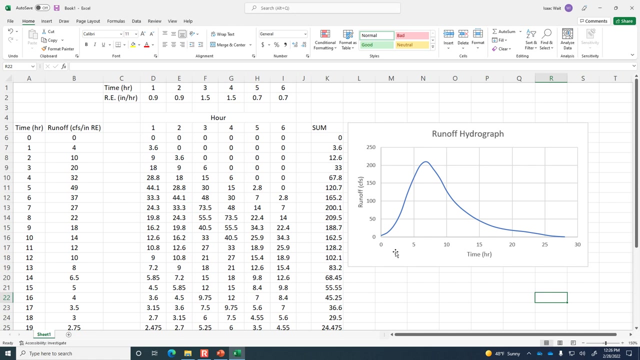 exactly to another spot, although we could take this unit hydrograph and transfer it exactly to another spot, although we could take this unit hydrograph and transfer it. Thank you, All right, so what we will expect is that this watershed is going to experience a peak. 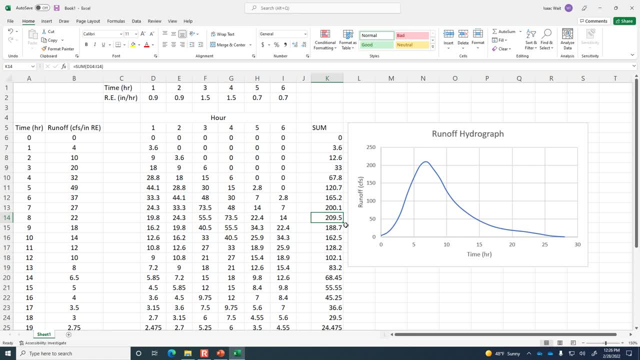 outflow of about 210 CFS for the storm event that we see Now. at the beginning of this example, I told you to keep in mind the issue of prior conditions, And so if you were going to predict, how might you expect the second hour would be different from the first hour? 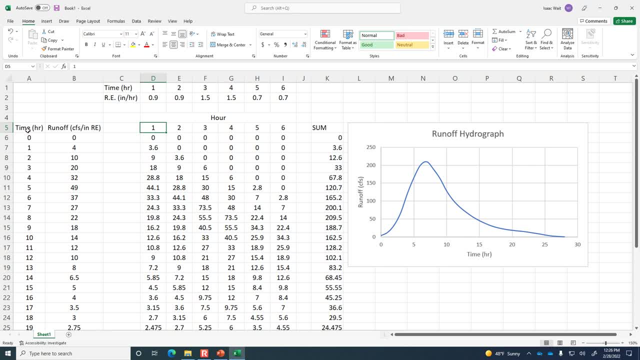 Like the runoff hydrograph says that one inch of rainfall excess would cause this response. But just think directionally. If you had this, for you know, you had the inch of rainfall excess in one hour and then you had another hour after that with the same inch of rainfall excess. 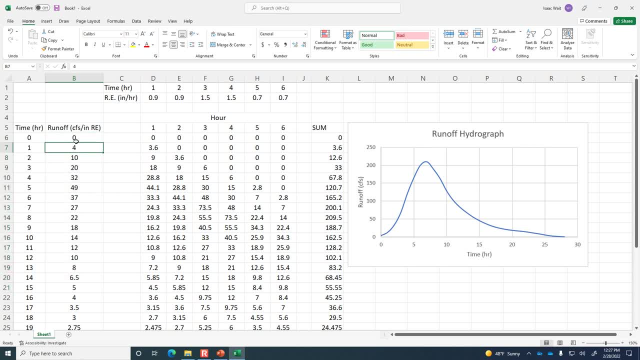 how would you expect the second hour of runoff to be different from the first? It would be greater because the rates of infiltration and all of that are going to be reduced. So maybe we're already accounting for that when we quantify the rainfall excess, You know, because remember that excess says by definition that infiltration has been accounted. 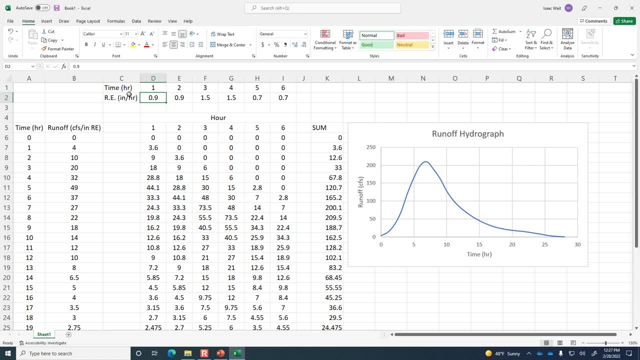 So probably what we would, rather than changing the hydrograph. what we'd want to do is say: well, is it really going to be the same 0.9 inches of rainfall excess for the second hour? You know, if we have two hours of the same amount of rainfall. 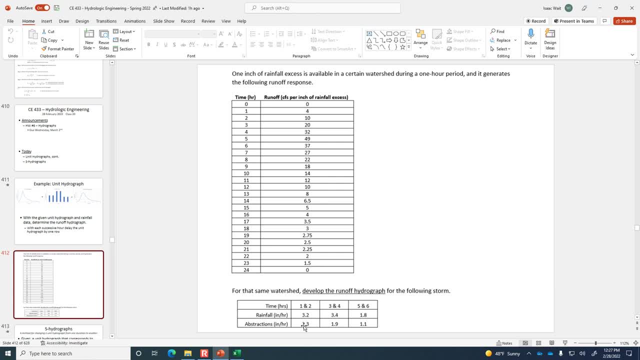 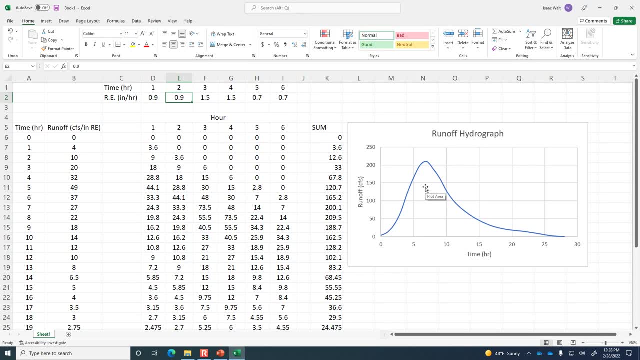 wouldn't the abstractions be less in the second hour? So we might be able to fine tune what the overall runoff hydrograph looks like by focusing in on that, But as far as how to apply it, we're not going to be able to do that. 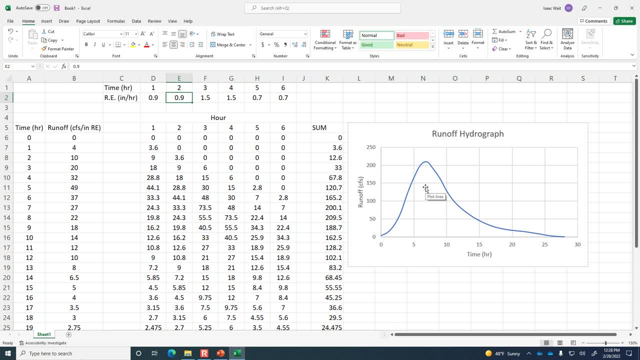 But as far as how to apply the method according, you know, like the textbook approach to applying the runoff hydrograph, the unit hydrograph, the key idea is that we're staggering in each successive hour by one additional row, So you can see that the leading zeros at the head of that column keep increasing by one with each successive pulse. 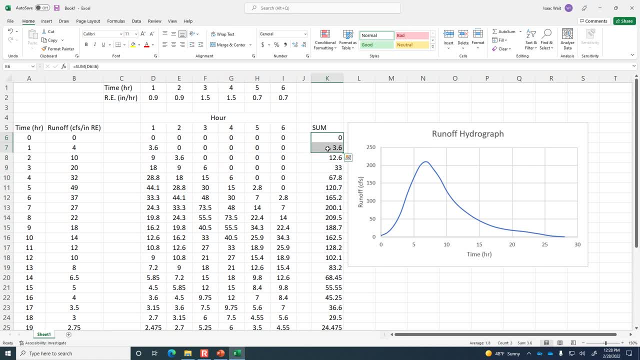 And then we add them all together in this column on the right side. Does anybody have questions on how to apply the method? No, All right, My suggestion is save this file so that you have it as a reference. I'll save it too, in case the power goes out, which it's done a couple times this semester. 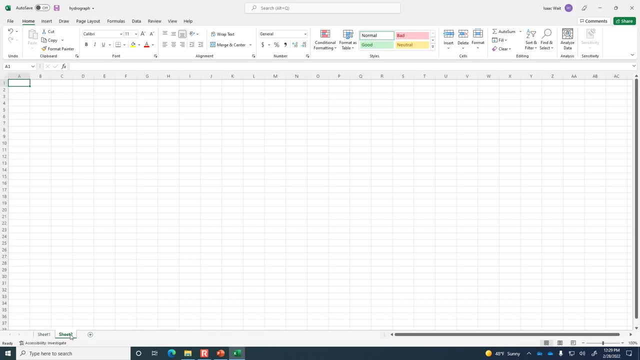 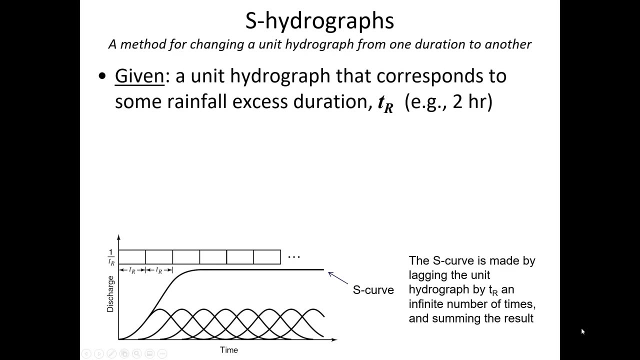 All right, And then create another tab, Because we're going to have to do this And then we're going to have an additional example in just a moment. Okay, Now the example that we just worked: we had a hydrograph that was for a one-hour rainfall duration. 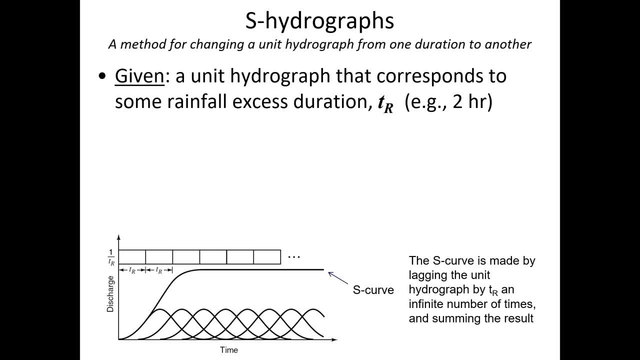 But what if we're interested to find out what is the watershed response for a different duration? We want to use the same unit hydrograph. So the S hydrograph method is a technique for changing a unit hydrograph And figuring out how its shape and timing is going to be adjusted if you have a different storm duration. 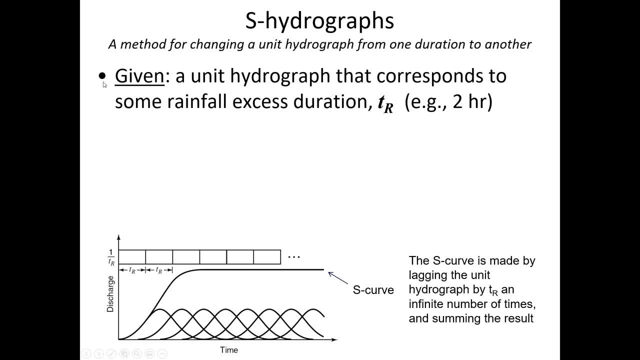 So let's say, for instance, that we have a unit hydrograph that corresponds to a duration of rainfall excess of two hours And we're going to call that storm duration T sub R. That's kind of the variable that our textbook assigns for the S hydrograph approach. 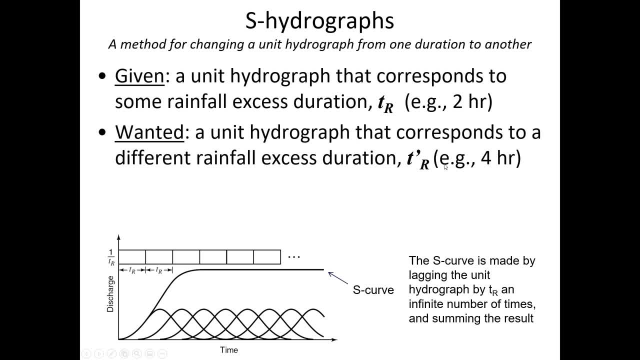 If we want to find out what would be, If we want to find out what would be the equivalent hydrograph for a four-hour storm- So it's the same unit of rainfall just spread out over a longer duration- Then what we'd expect, of course, is that the peak rate is going to be lower. 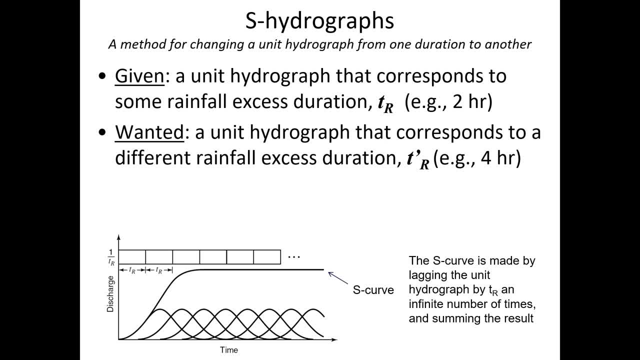 And it's going to arrive slower, But how much So? that's what the S hydrograph method does And the technique that it uses. the reason why it's called an S hydrograph is that you repeat the normal unit hydrograph system. 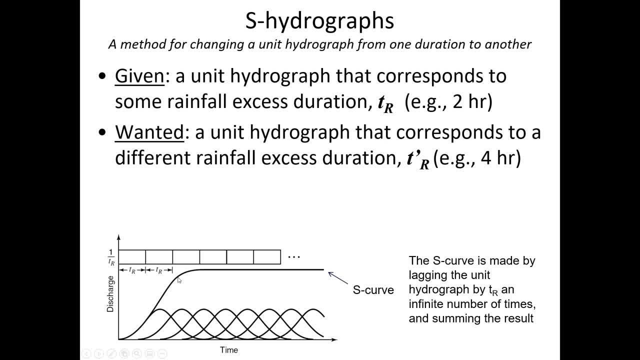 Several times together And you add up all of those unit hydrographs And the S curve is the resultant of adding all of the delayed given unit hydrographs. And then you go through a process of delaying the S curve and dividing by the ratio of the two durations to find out. 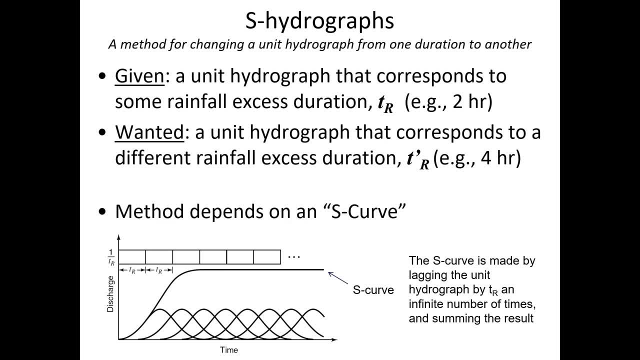 the new unit hydrograph for the longer storm. So that's what we're going to do. I'm going to illustrate and I would recommend that you follow along, Just so that you've got a reference of your own that you can go back to when you're working on the homework. 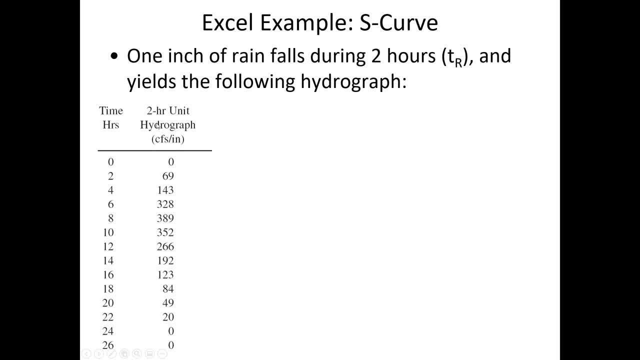 We're going to start off with this given unit hydrograph. that was an inch of rainfall excess that fell over a two-hour period. So from time zero to time two we had one inch of rainfall excess And then this is the hydrograph that it generated. 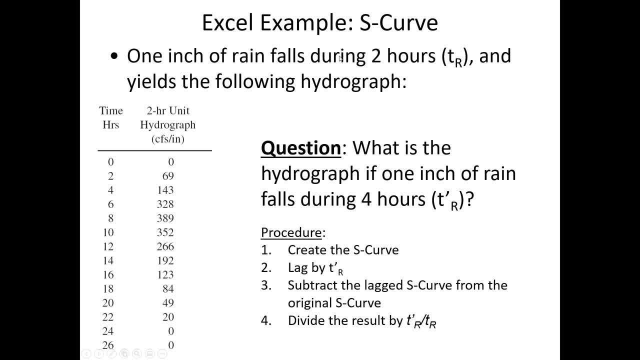 So T sub r is two. And what we want to do, we want to know, is what is going to be the equivalent hydrograph for the same inch of rainfall excess but with a longer storm duration. So T prime r is four. So just to summarize the procedure I'm going to go through, 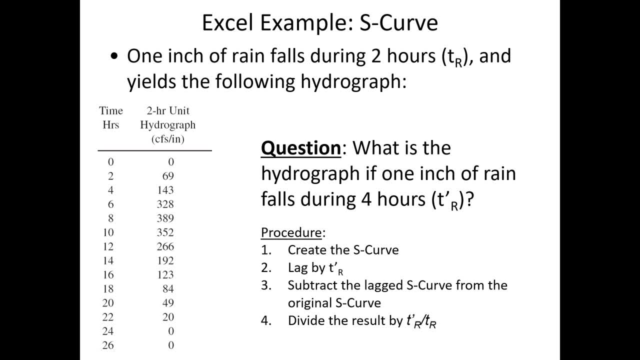 first of all, we'll create the S curve by repeating this given hydrograph over and over again, with no adjustments, just copying it and repeating it, And then we're going to lag the S curve by T prime r, which you can see here is four hours. 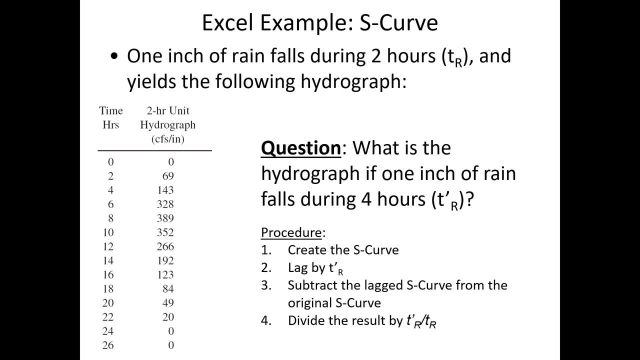 So lagging it means we just create a copy and we paste it four hours down, Then subtract the lag curve from the original S curve and then divide to find the height of the peak by the ratio of the desired to the given storm duration. All right, 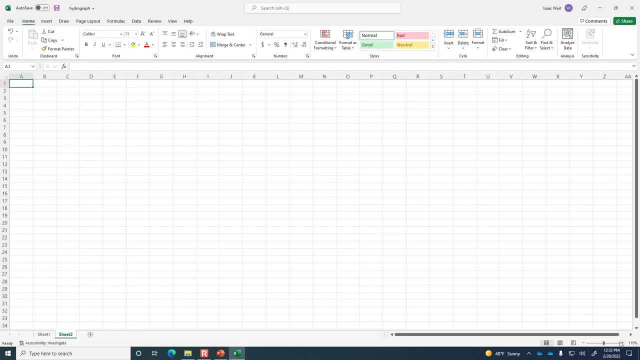 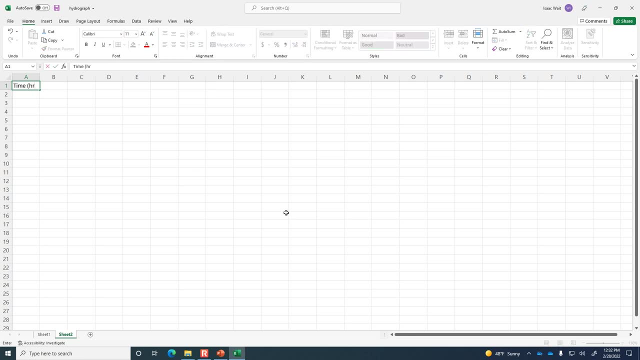 So we're just going to start with this blank worksheet and we're going to have to key everything in here manually. That's fine, It's not too bad. So time in hours. So time in hours is what we're starting with. And then the two hour unit hydrograph. 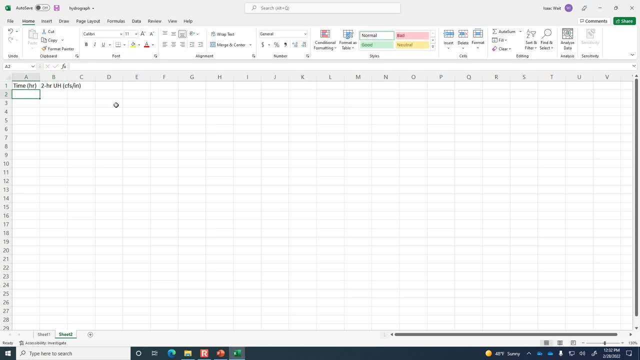 which has units of CFS per inch of rainfall excess. So just, first of all, digitizing the given data. So we had zero, two, four, and it goes through a period of 24 hours, All right, And then the given runoff was zero CFS. 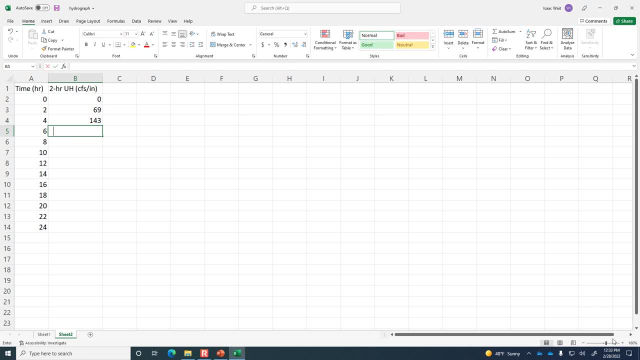 149, CFS, 143,, 328,, 389,, 352,, 266,, 192,, 123,, 84,, 49,, 20, and zero. So that's the given. So the first step that we're going to apply here is create the S curve. 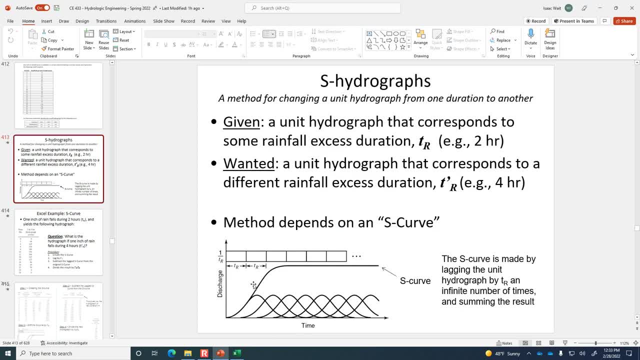 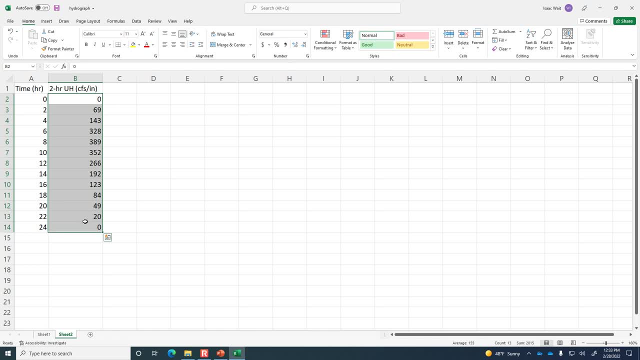 And the way that we create the S curve is that we just repeat the given unit hydrograph over and over again. So I'm going to take the given unit hydrograph and repeat it with the same technique that we did with the other unit method. 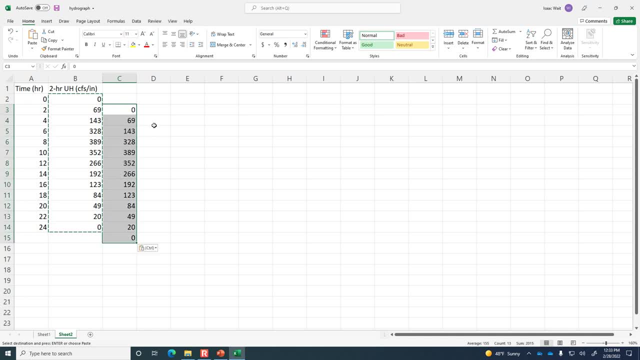 where I am pasting it a row down and then paste it a row down again and again. So I'm just doing control V to paste over and over again, paste it, paste it, paste it. And so in this case, I think, like, how many times are you going to paste it? 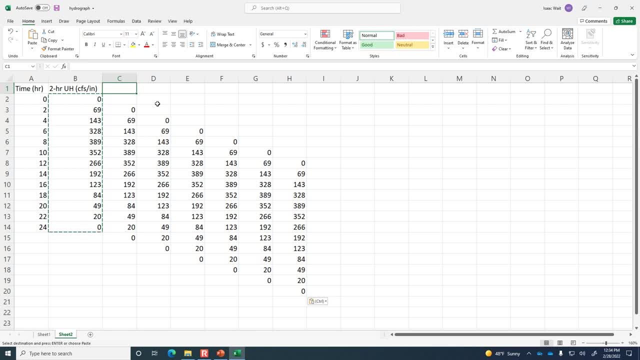 You don't necessarily know- until you have created the S curve, because we want it to achieve this stability for long enough that we can subtract out the S curve again. So just to make sure we have enough, I'm going to do 12 columns. 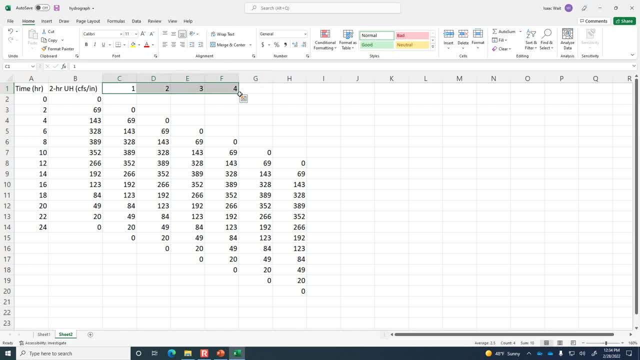 One, two, three, four, 12 columns. One, two, three, four, 12 columns. One, two, three, four, 12 columns, And, of course, if it doesn't work. that's a very easy task. 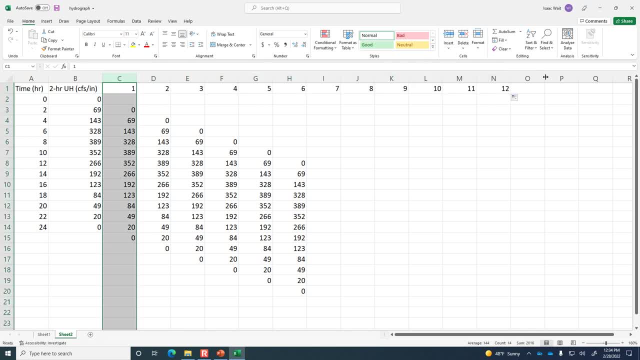 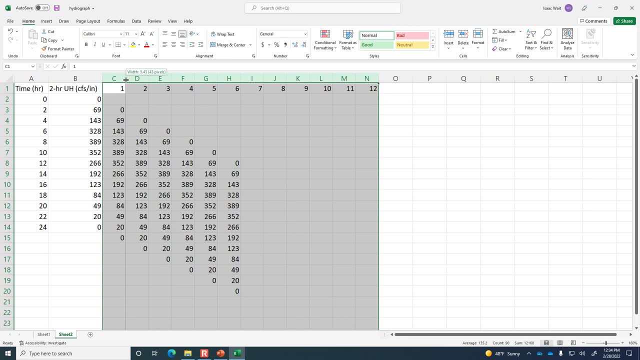 And, of course, if it doesn't work- that's a very easy task- If it's getting too big, you can change the width of these columns, just to make sure that we're fitting it all on the same page. If you highlight the columns and then change the width, there we go. 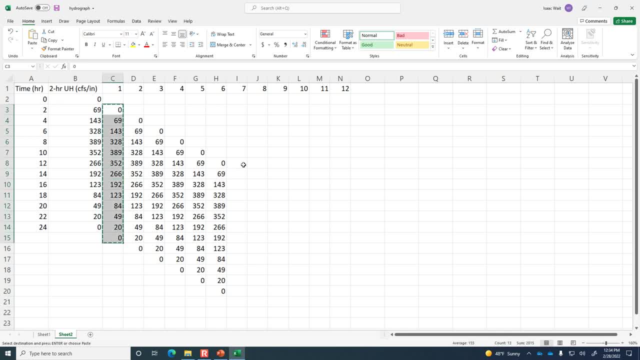 So let me continue pasting a few more times, All right. so the first part of the lag is just to repeat the unit hydrograph with a delay of two hours each time, and then we want to sum it all together, So it is the sum of all the columns to the left, and you don't have to put zero in the cells that have nothing in it. 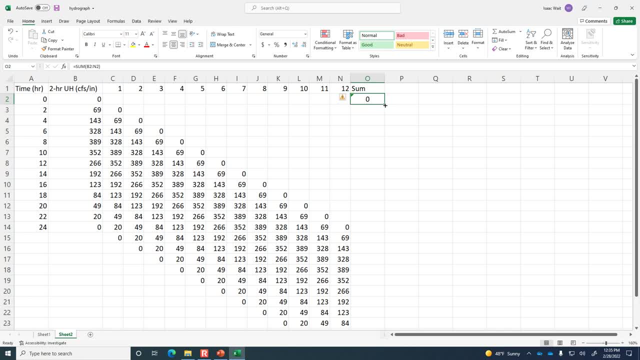 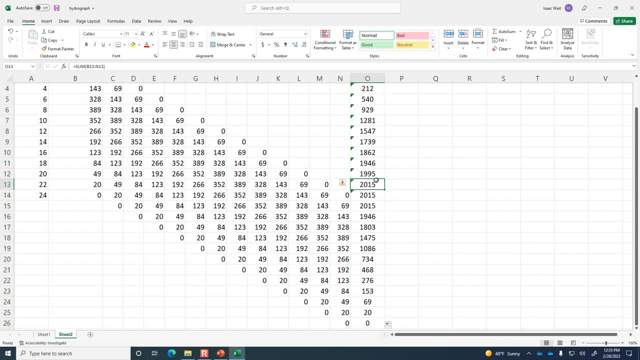 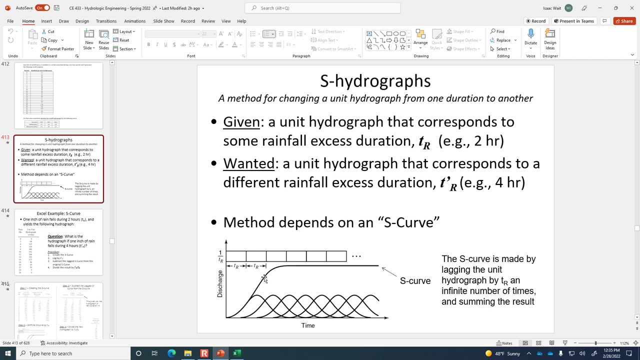 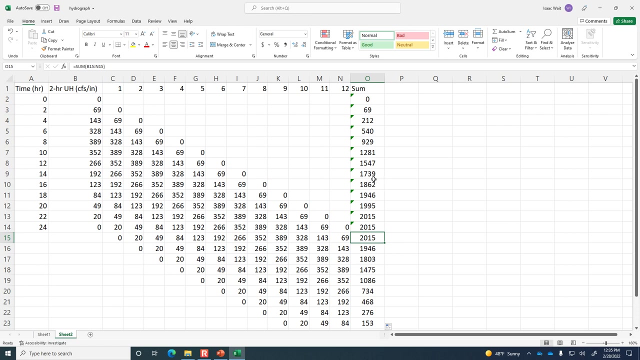 It'll still read that as zero. All right, so we've done it enough times- that it achieves kind of this upper asymptote, 2015 CFS, and that's kind of this part of the S-curve. And if I repeated it more and more times then this would continue. but I don't necessarily need to have an infinite number of columns. 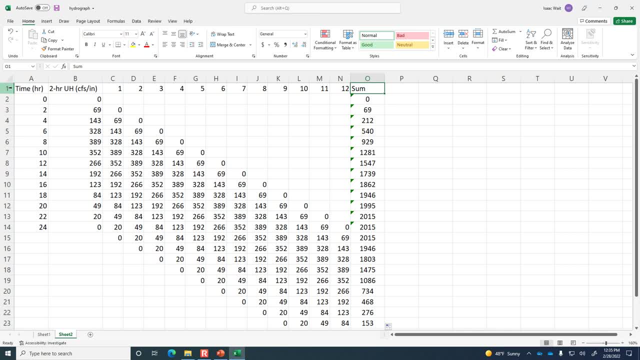 I think this will be enough. Okay, so this is the S-curve. Let me just create another row there so that we can title: this is the S-curve. And then we want to have a lagged S-curve and the instructions tell us to lag it by D prime R. 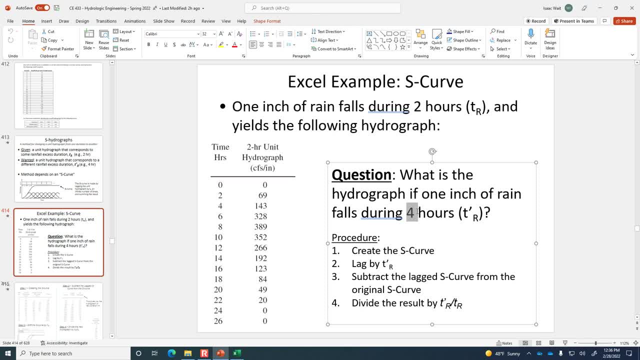 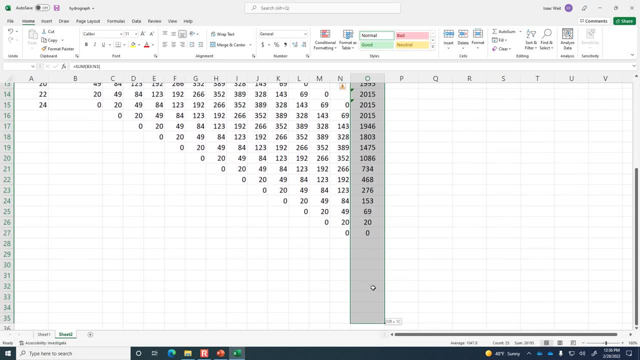 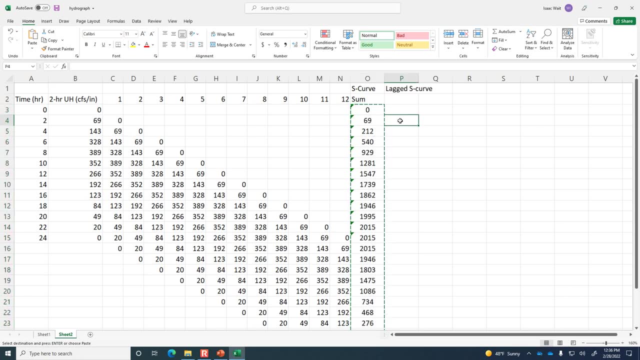 So lag it by the desired duration of four hours. So I'm going to copy this same curve. so I'm just going to highlight it here. Got it highlighted. copy control C. Now where to paste. If I followed the same thing of just pasting it in the next row, then it's only been lagged by two hours. 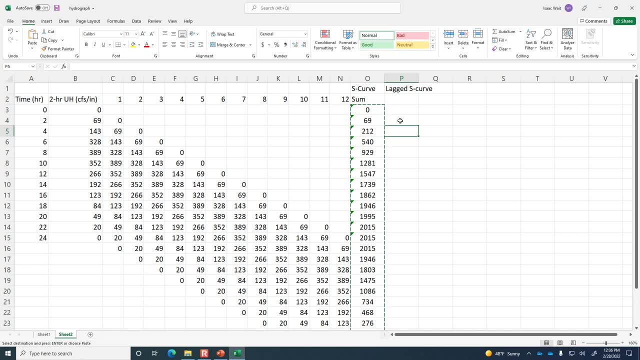 So that's not enough. I need to lag it by four hours, So I'm pasting it down here. I need to paste values because it was a formula. This is a tricky thing. Look at what I have in here as a formula. 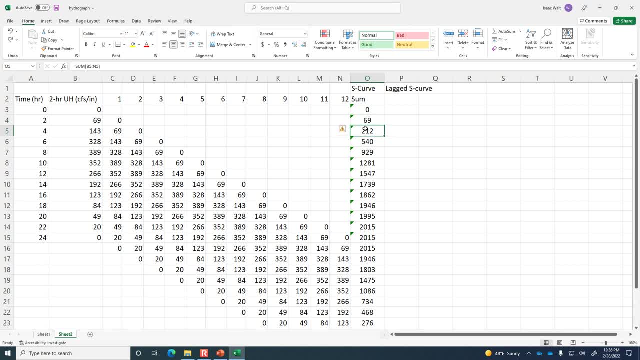 Sum of B3 through N3. And so on. So these are formulas. So when I highlight it, if I do control C and then if I paste, just the default paste is to paste the formulas, But I don't want to paste the formulas. 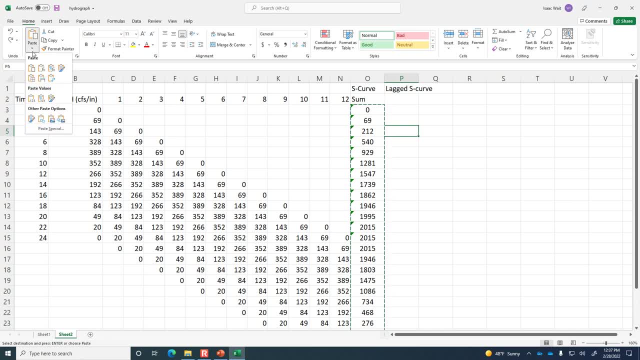 I want to paste the values, So I'm going to go paste values so that it pastes the numbers themselves and not the equation. So just to make sure we're all on the same page. we're seeing the zero four hours after it occurred in the F. 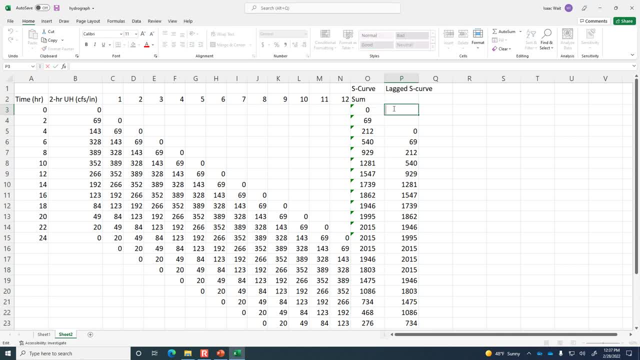 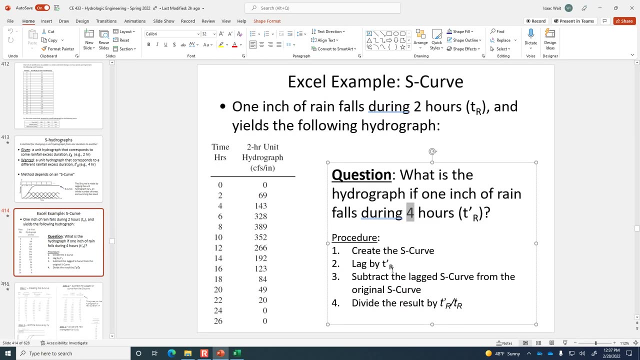 In the S curve. So the original S curve had that zero at time zero. We see it at time four. And then 69 CFS was at hour two. Here our 69 CFS is at hour six. So we have successfully implemented this. lag by T prime R. 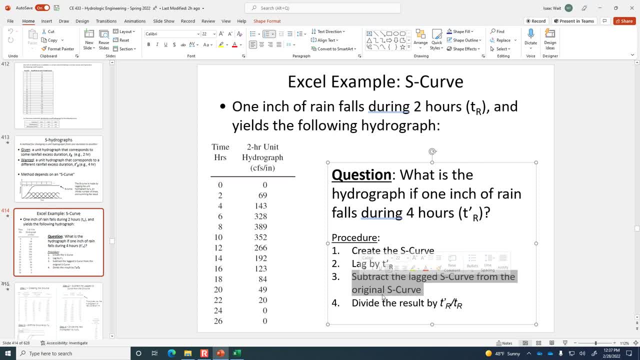 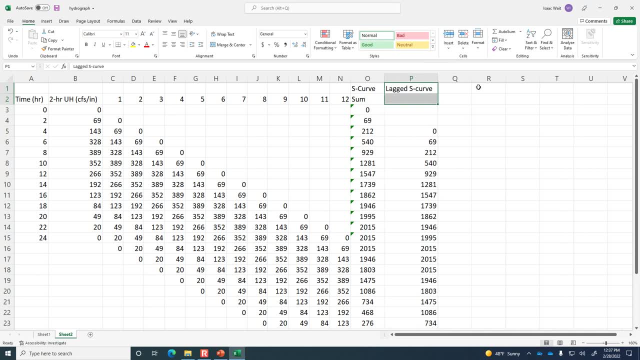 Okay, so step three is to subtract the lagged S curve from the original. So here's the original S curve, Here's the lagged. So our next one is the lagged four hour hydrograph. So subtract equals this minus that. 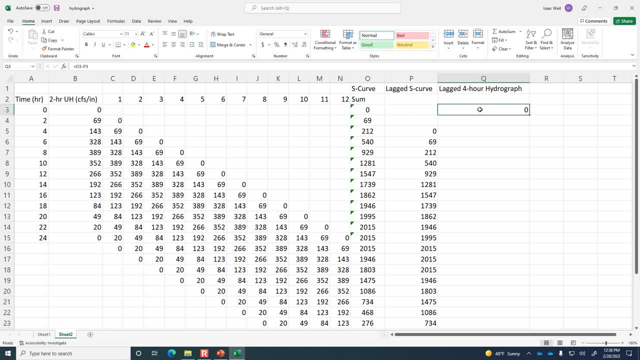 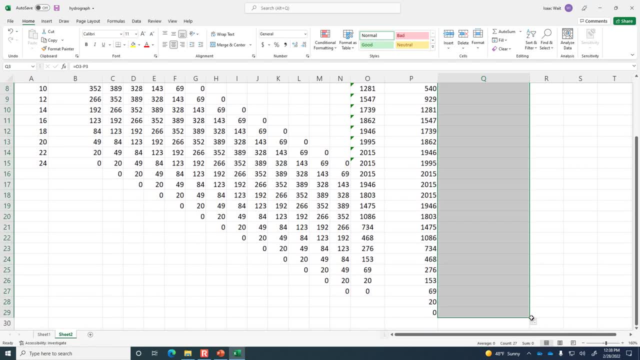 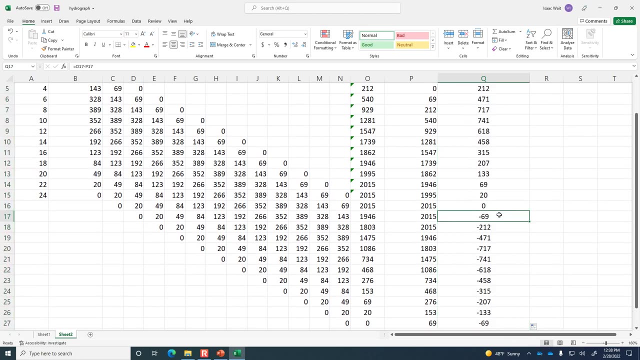 The original minus the lagged. Okay, Now we've got some spots where it goes negative and all of those can just be overridden as zero. So we don't have negative flow rates after a certain time, It's just the watershed is drained and it goes to zero. 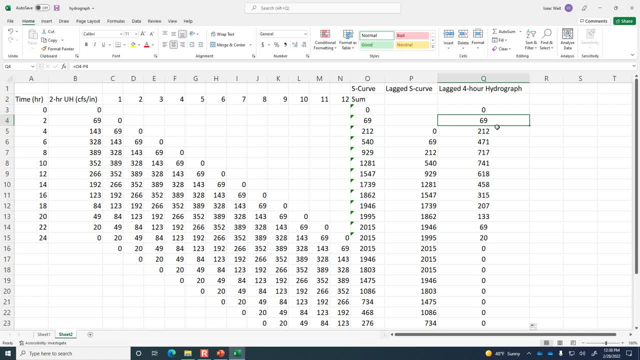 Okay, so here's our lagged four hour S curve, And the only other thing that we have to do is we have to divide the lagged four hour S curve By the ratio of the times, because, remember, this is an inch of rainfall excess that spread out over four hours instead of out of two. 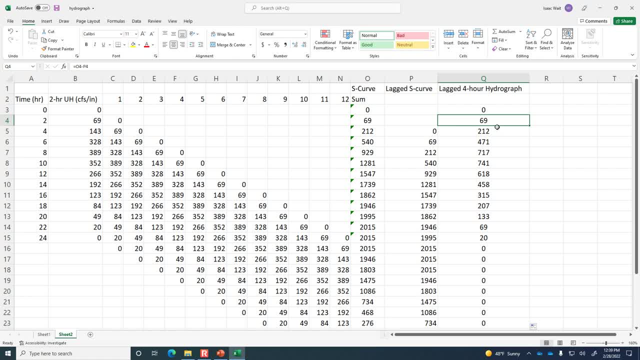 So we're going to see lower peak flow rates And right now this would suggest that the peak flow rates are higher. Look at the original. This is an inch of rainfall excess and the peak that we saw was 389 CFS per inch of rainfall access. 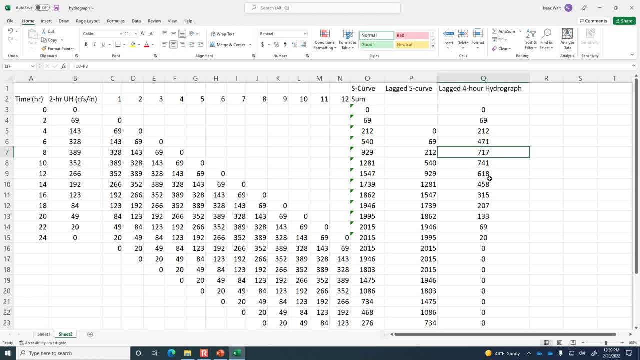 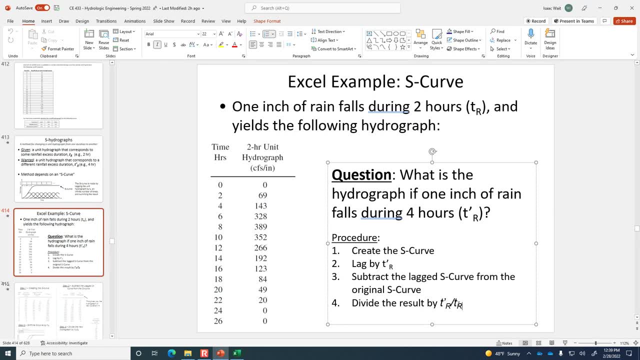 And that was here at time eight. Well, so far, this is saying well, it would be higher flow rates. And so this last step that we're applying: divide the result by T prime R, divided by TR. So T prime R for us is four hours. 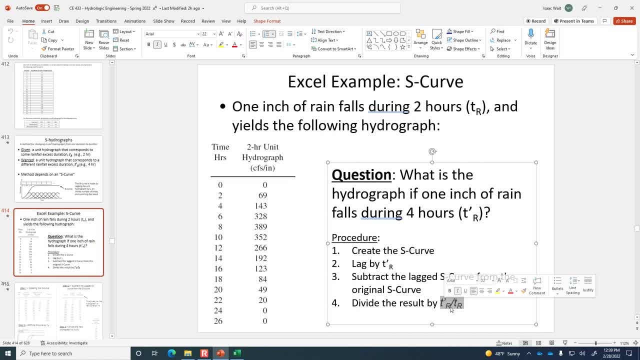 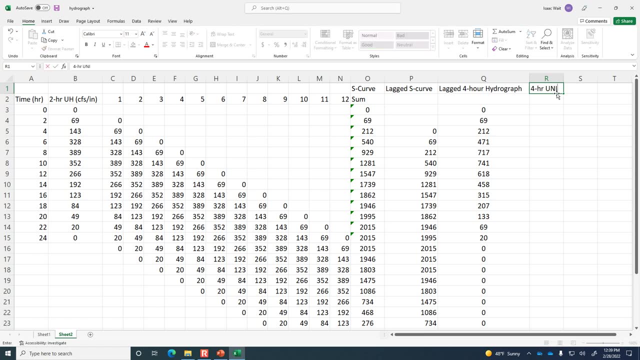 TR is two hours, So we're going to divide by two, So I'm going to call this final column here the four hour unit hydrograph. Okay, so it is each of these amounts divided by two, And it's the times still apply. 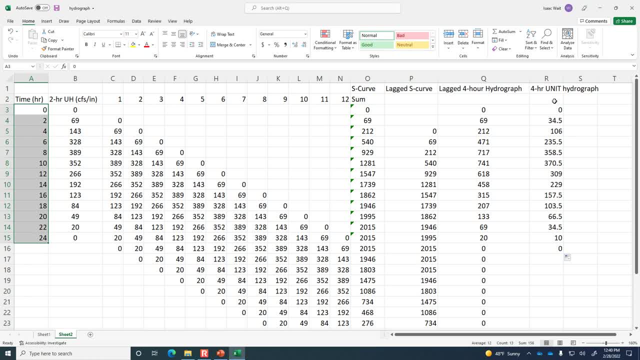 But the let me highlight this so that we can see the final hydrograph, So the four hour unit hydrograph, instead of being 389 as the peak, the peak is 370.. And you can notice that it also is an hour later. 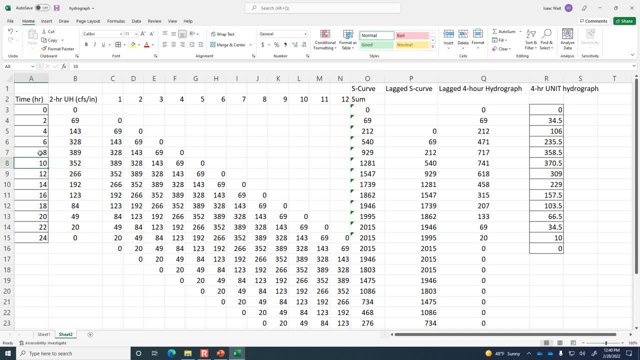 Well, not an hour. It's at hour 10 rather than at hour eight, So it's been delayed into the next time increment because the rainfall itself was spread out over a longer duration. So we still it's not like you won't see any flow during the first four hour block. 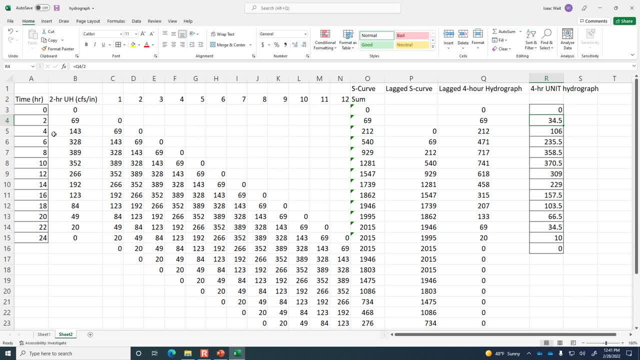 There is still a little bit of runoff observed at hour two, But it's just the. because the rainfall is spread out over a longer duration, the peaks are lower And delayed a bit. So that's the S hydrograph method, And combined those tools are surprisingly valuable. 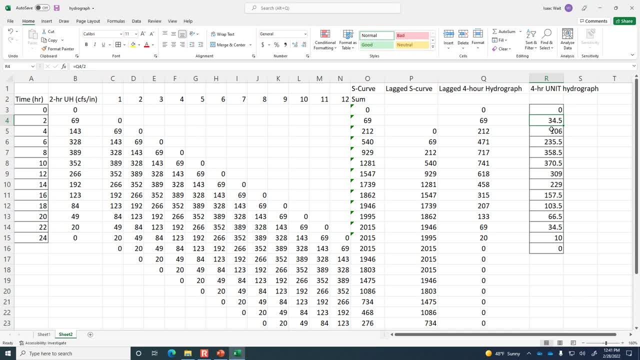 These techniques are going to be kind of working in the background when we get into these really sophisticated watershed models. They're built on the fundamental principles of a unit hydrograph lagging the unit hydrograph based on what kind of rainfall is going to be. 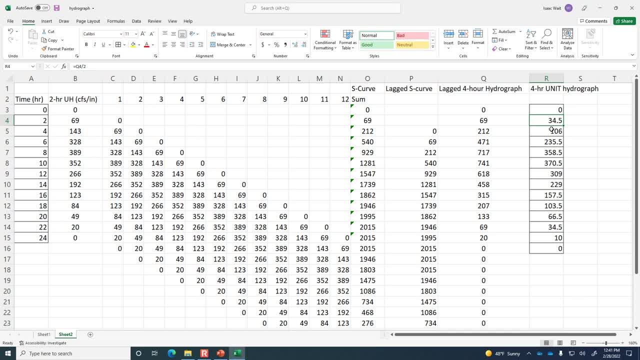 And what kind of rainfall is going to be And what kind of rainfall is going to be And what kind of rainfall is observed. breaking up the rainfall experience into tiny little time pieces And kind of numerically integrating what happens through the watershed. Any questions on the S hydrograph approach? 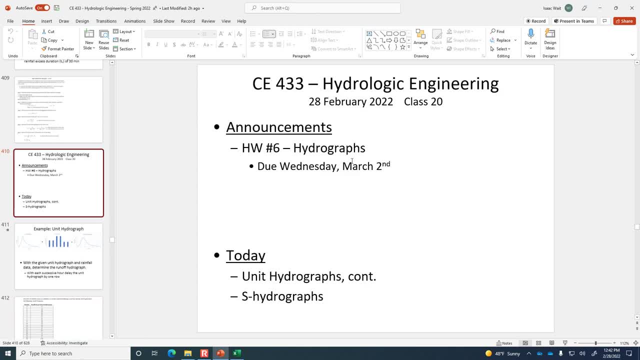 All right, That's all I have for you today. Remember that this homework six is due on Wednesday, So if you have questions as you're working on that, please let me know and I'll be happy to help you out. See you Wednesday. 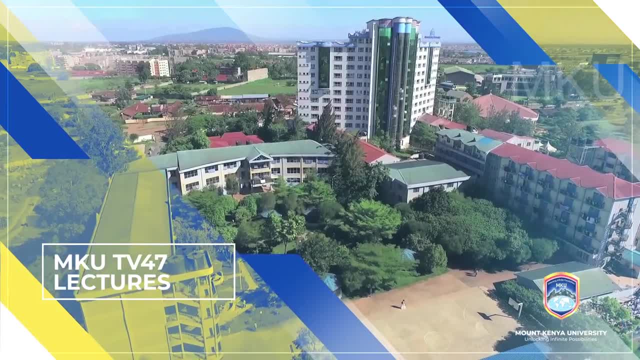 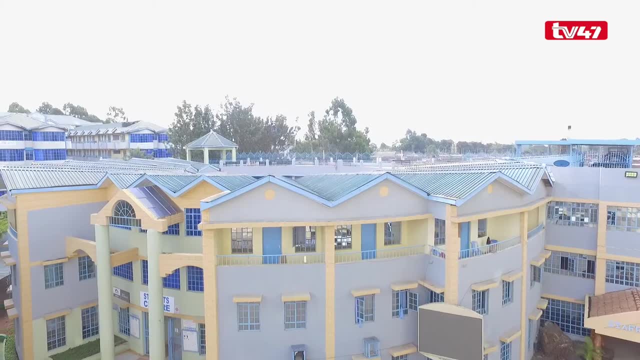 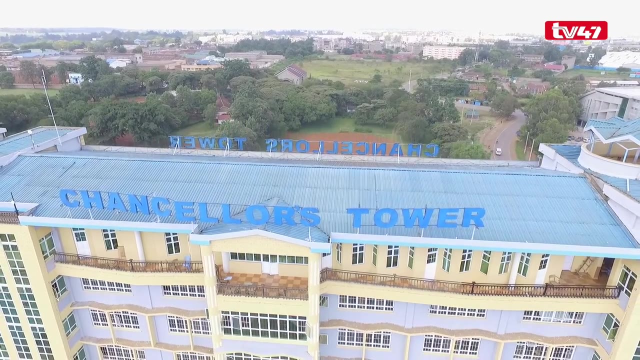 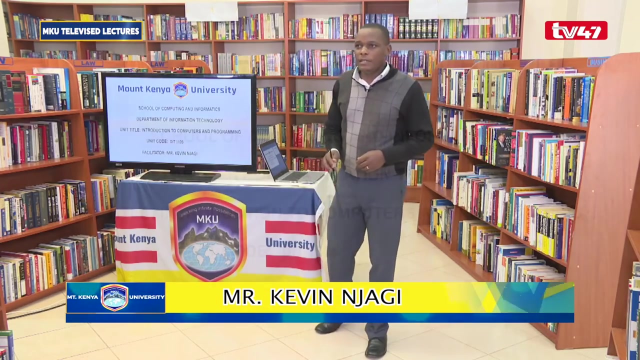 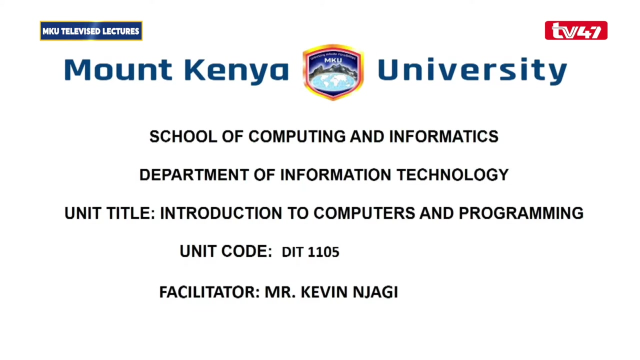 Hello everyone, Welcome to today's lesson. I'm Mr Kevin Jaggi from the School of Computing and Informatics. Today's unit is Introduction to Computers and Programming And by the end of this particular lesson you're going to understand what is a computer, what makes.